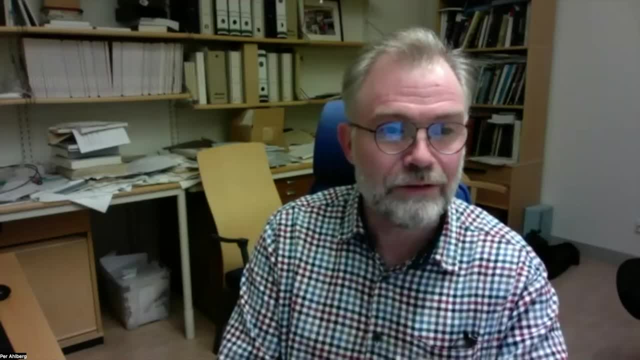 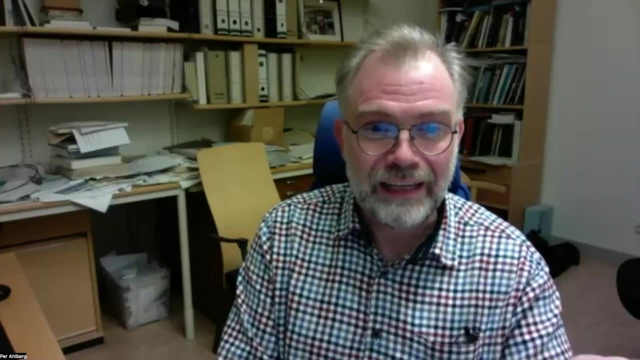 And, by the way, I know that different people are using they're using the term hominin in slightly different ways. As I'm using it now, I'm really talking about the human total group, In other words anything upstream from the human chimp lineage, split, that's, on the human lineage. 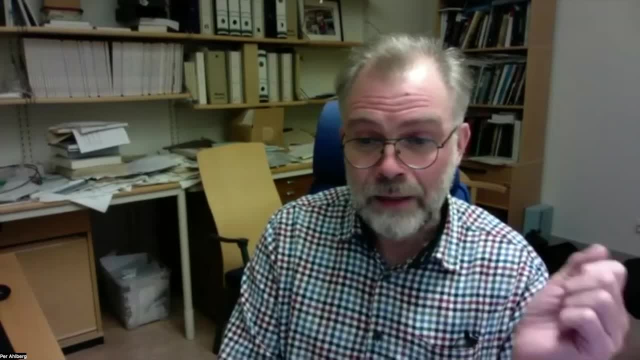 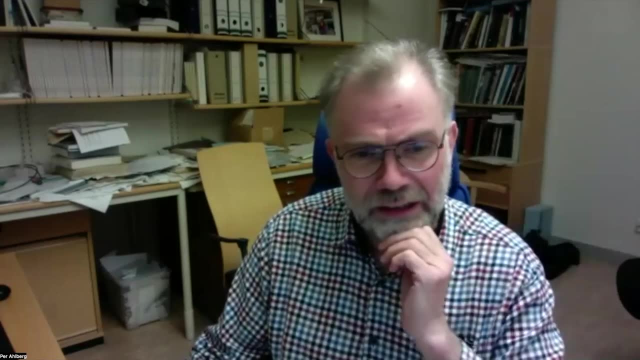 STEM group members, of course we're talking about here right down the bottom end, But anyhow. so they had what they believed to be hominin footprints from the late Miocene. Well, that's kind of exciting. But what was particularly kind of startling? 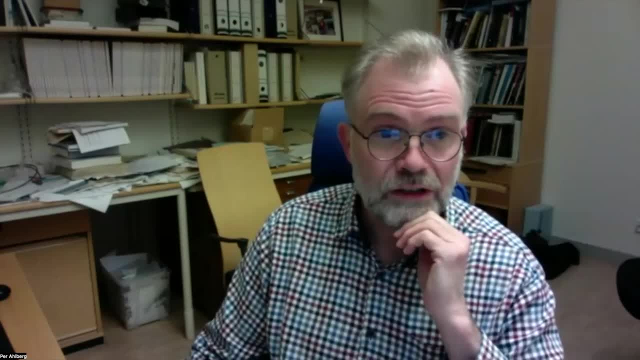 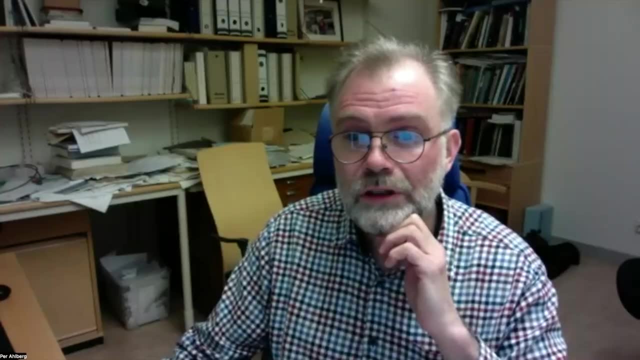 Yeah, Yeah, Yeah. What was particularly kind of startling about this is that we're not talking about Africa now, but from Western Crete. I can in fact put on an image. Let me see one moment. That would be perfect. 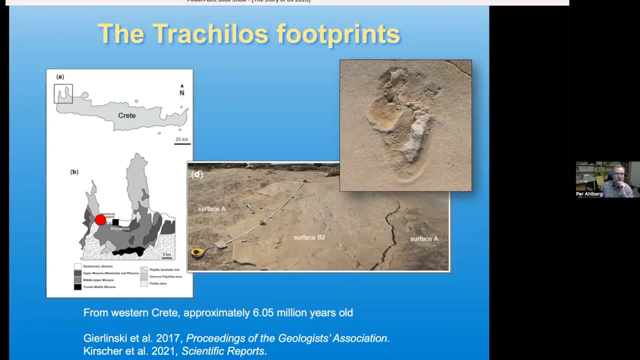 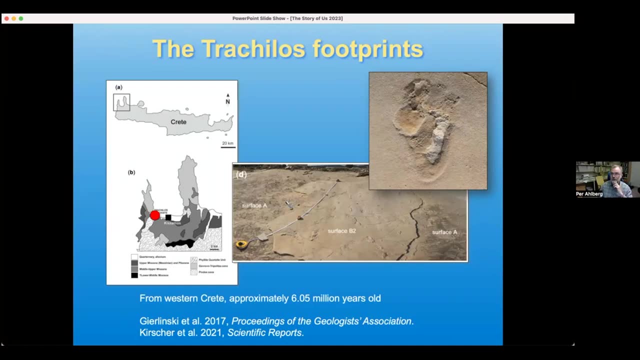 Okay, Mike, I should shrink suitably into the background and you should now all see an image, Blue background. it'll say the Trachylus footprints. it'll say, and I'll have some pictures. Does it show up? 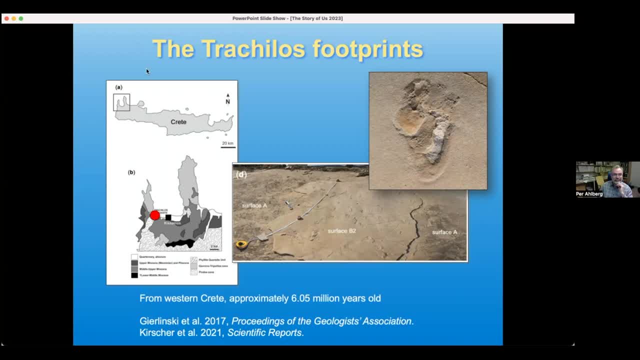 Okay, super stuff. So what you've got here is a map of the island of Crete. I take it you can see my pointer moving around. yeah, Correct, And over at the western end of the locality called Trachylus in late Miocene strata now dated to about 6.05 million years. 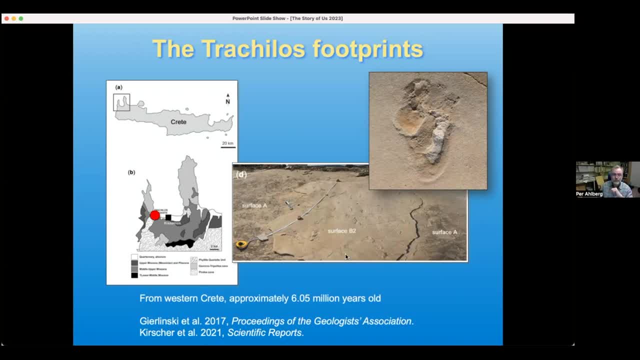 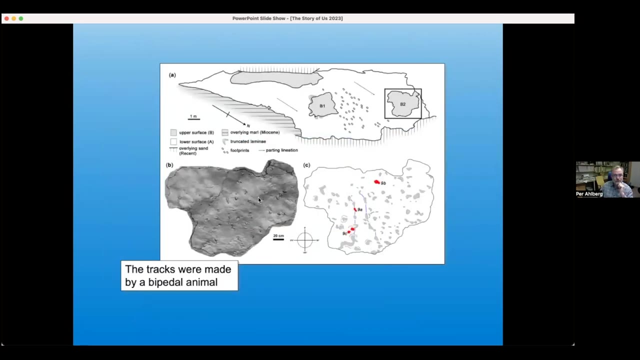 in what's otherwise a very shallow marine sequence, we have a little emergent episode with basically probably a sandbank in an estuary or something like that, with really rather beautifully preserved footprints. This image shows the black and white image, so it's not a photo but actually a laser surface scan of the main footprint surface. 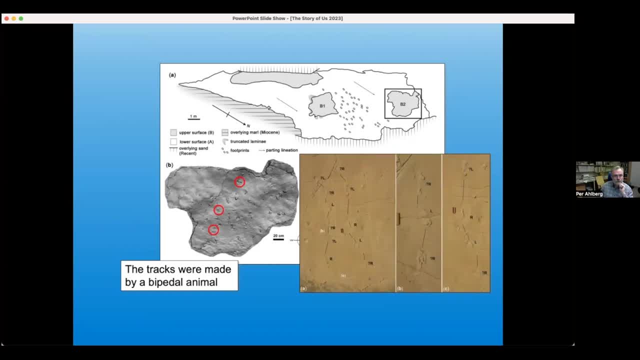 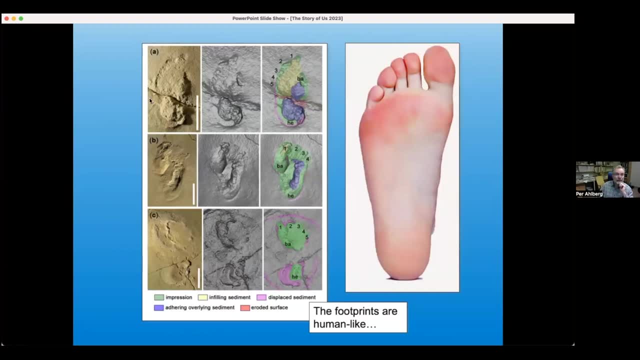 That's not very informative, but those three red rings. there are three of the best preserved prints which you will see in the next image here, And in each case here you've got a photo on the left, a scan image in the middle and a color-coded interpretive scan image on the right. 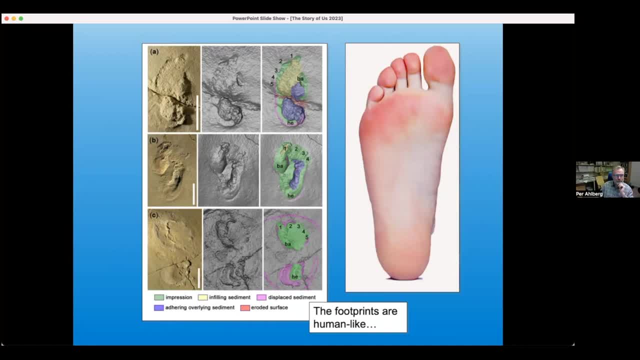 And, as you can see, they're really quite distinctive footprints. The size of these is a little bit variable, but they're typically of the order of about so. so you know, modest-sized feet. What's very interesting about them is that – I should say, by the way, so you know, I got drawn into looking at this stuff. 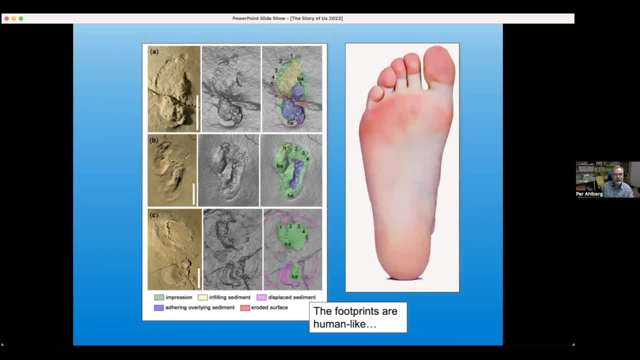 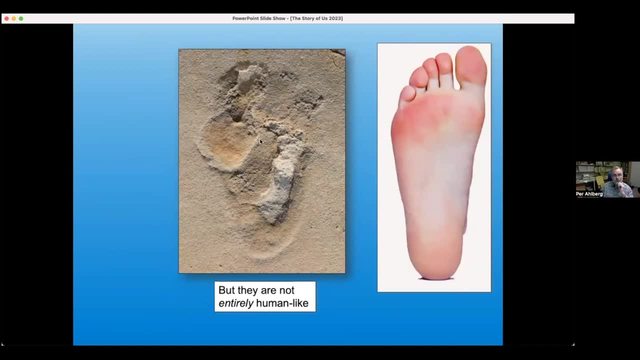 and I could only concur that, yes, they do indeed look very human-like – but what's interesting about them is that they're not entirely human-like. So here is one of the best preserved ones. You can see, by the way, it's a really, really beautifully preserved print of very sharp little expulsion rims. 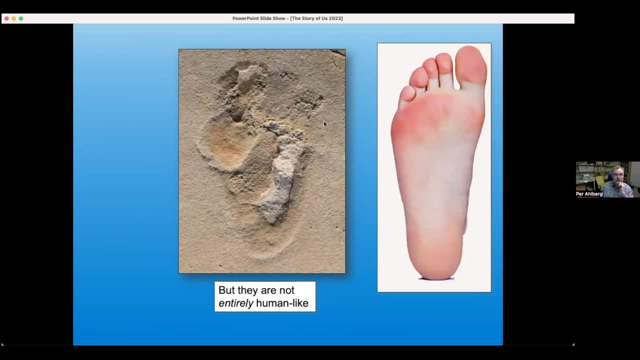 This is on a sand surface that evidently dried not that long after the print was made and you have these sort of pull-up features left by – where the foot sort of adhered to the surface before it was pulled off – big toe there, obviously, and some of the other toes there. 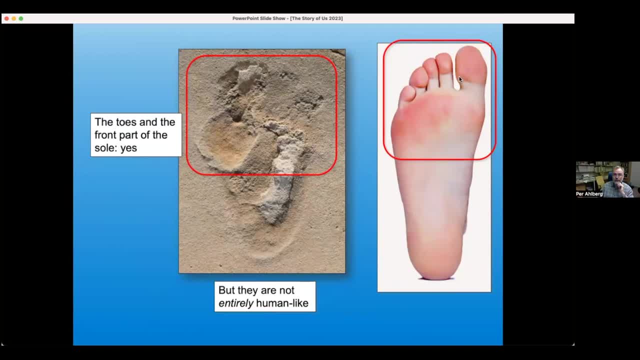 Now look at this. So this is a human foot And, by the way, as I'm sure the viewers appreciate, human feet have a really, really large footprint, really distinct, really kind of unique morphology among, well, actually among, like everything there. no other vertebrate has ever developed feet that look quite like ours, which, of course, is. 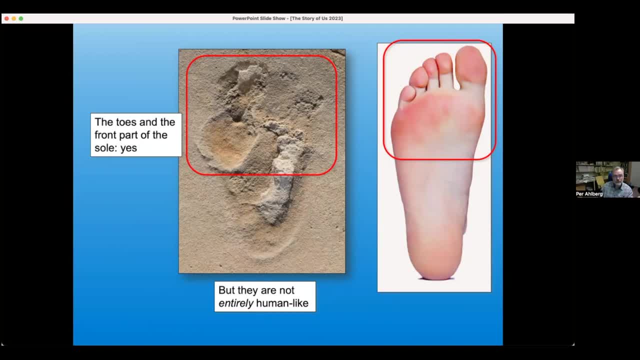 quite interesting, then, in terms of understanding their evolution, but also neat in terms of the the distinctiveness of fossil, human or near human footprints. so what have we got here? well, we've got a front end that looks very like human foot. you've got this lovely ball. it's really kind. 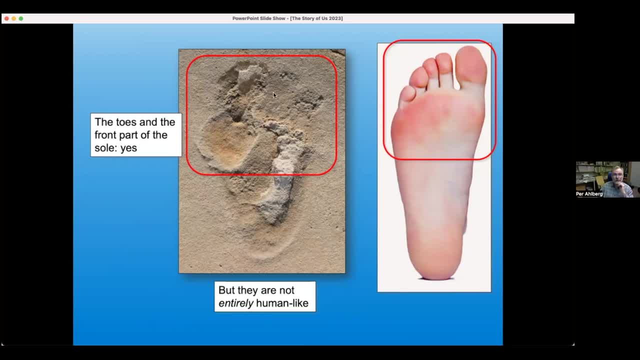 of ground into the sediment here and you've got a big toe immediately adjacent to the, the next sort of index toe, i suppose you could say. very much like in a human foot, but as you can see already, the back end's not the same. back end's much shorter. the heel isn't bulbous like in us. 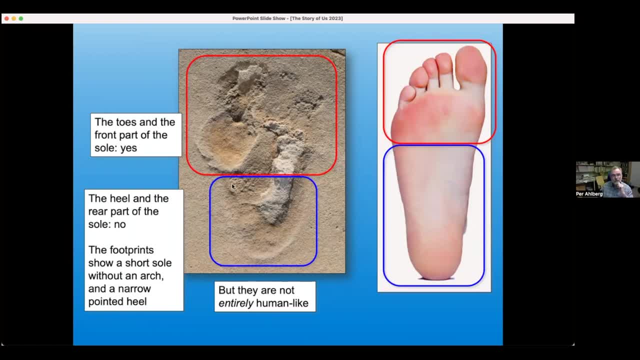 and while there's a degree of asymmetry to the print is suggesting that our friend here is putting more of more weight on the outer edge of the foot, hence the pull-up structure. here there's no real arch, it's essentially kind of a flat foot, um, and so this, of course, is kind. 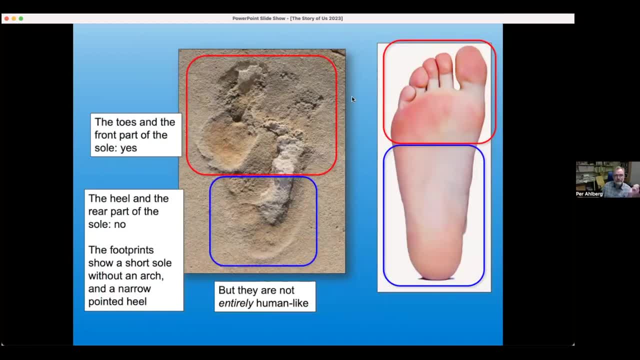 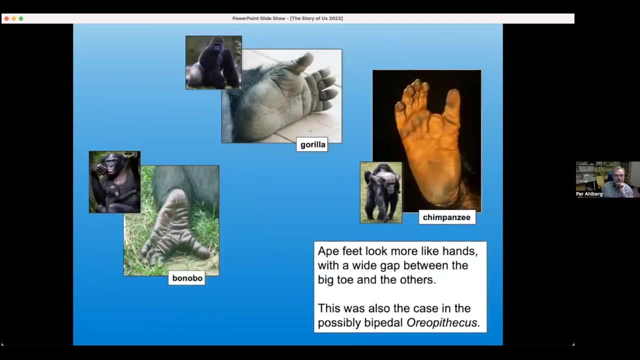 of lovely, because what it, what it gives you, is kind of a front end human foot attached to the back end of a more sort of generic ape-like foot, if you will. if you look at the feet of modern apes, because obviously you know, you might look at this foot and think, well, okay, what might be going on? 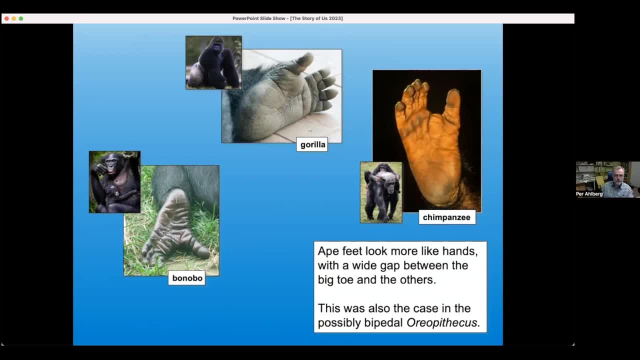 here. you know it's a. it's some sort of mammal that's walking around, doesn't have claws. primate interpretation seems like a good bet, but could it just be some sort of ape then? um, but if you look at ape feet, there we've got bonobo, chimpanzee and gorilla. um, what? 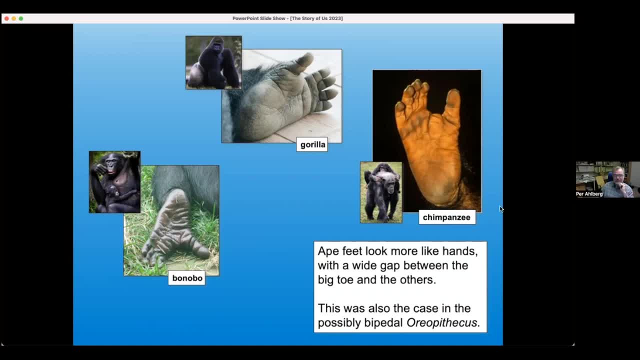 all of them show is they're all fundamentally somehow hand-like. you always have this big gap between digits one and two, and you can also see that it's not just that, but digit one, the big toe, is set a little, as it were, down the side of the foot, and it's not just that. it's not just that, it's. 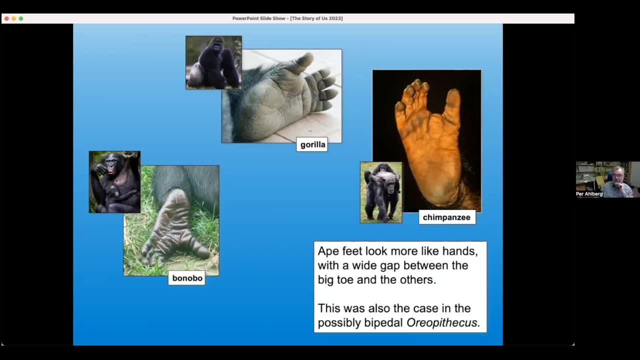 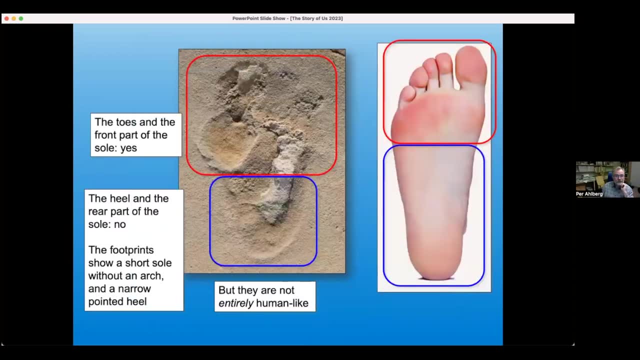 the side of the foot so that even if you were to pull this in, it would lie a little ways back some of the way my thumb does here, whereas if we go to these footprints again, you can see that the big toe is set on the front of a transverse edge of the sole in a very human sort of manner. 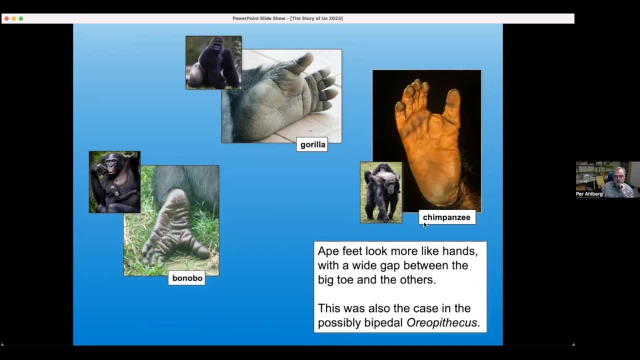 um, but the back end of the foot looks, you know, quite plausibly like what we see in the trackless prints. interestingly, there is a fossil myosin ape from the mediterranean region called oriopithecus, which has been argued by some to be bipedal. i think that's a little dodgy. but aspects of the 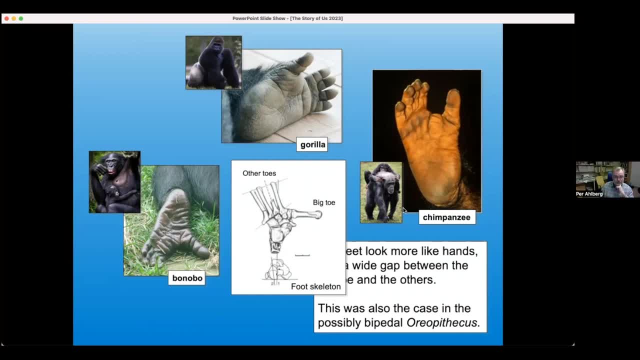 skeleton suggest it, but it still had ape feet. um, you've got this very. this is the foot skeleton of oriopithecus you see here, and the big toe. this is as preserved in the rock, and the big toe flares widely out from the other toes, so clearly it's doing a kind of ap thing. in fact, you know an. 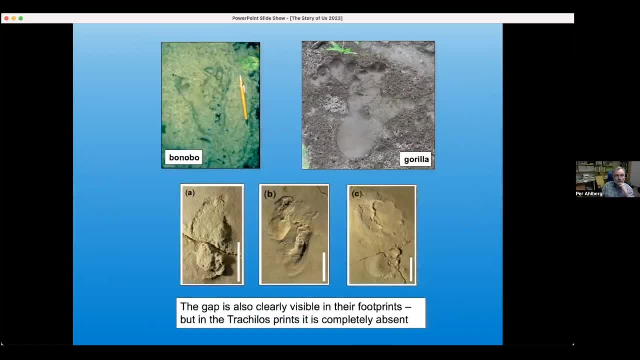 almost like a foot skeleton, but it's not a foot skeleton, it's a foot skeleton. it's a foot skeleton exaggerated way. and when you look at the footprint of living apes, there's a bonobo print and a gorilla print, both of these, by the way, from the wild, which i feel is of some importance, i mean. 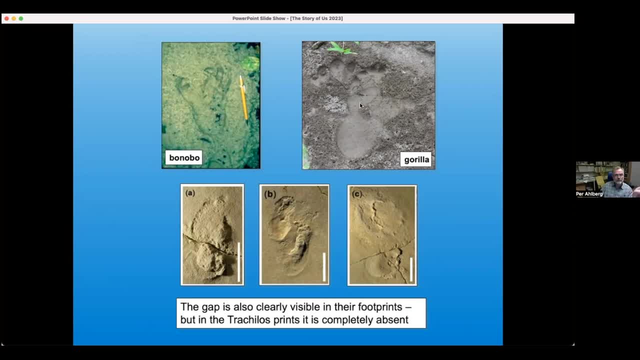 i always worry a little bit about what animals do in zoos, but these are, you know, bonobos and gorillas, respectively, going about their business in their normal environment. this is what their feet look like and you can see immediately that you have this very wide spacing, and you can see. 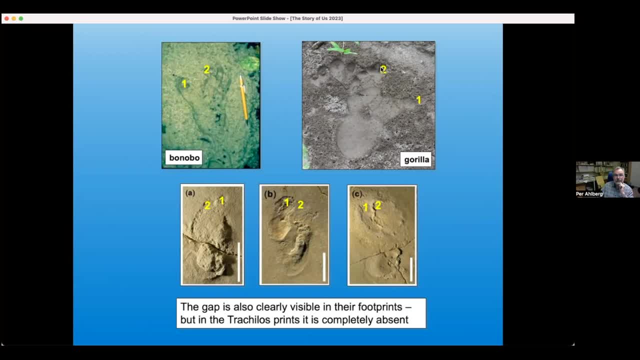 of the, the big toe print, and the, the, the index finger, if you like, index toe print, and then the other little toes around curling around, so completely different to what we see in the trachylos prints, where one and two are always tightly together, um, and it should be said that. 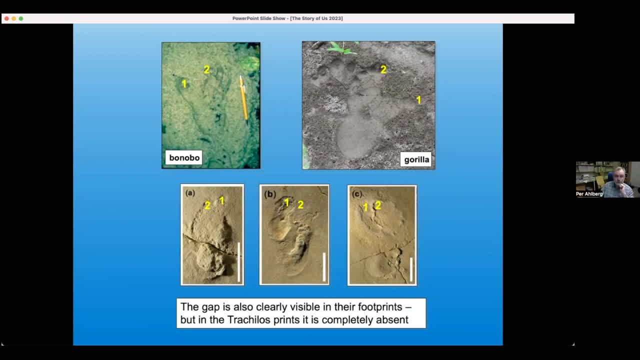 while these are the three best preserved prints, not one of the prints on that surface shows anything like a kind of l-shaped morphology. so even though the less beautiful prints, plainly, were made by someone else, they were made by someone else. they were made by someone else something where where digits one and two were held tightly together. so i looked at this and 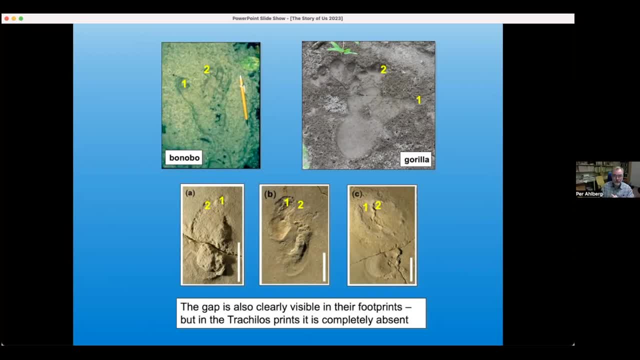 well, let me, you know, look, that kind of nails it. this is a derived character of humans that we don't see in in other primates. so we're, you know, we're within the human stem group here in some some little way up, which of course then becomes really interesting, given the great age of these. 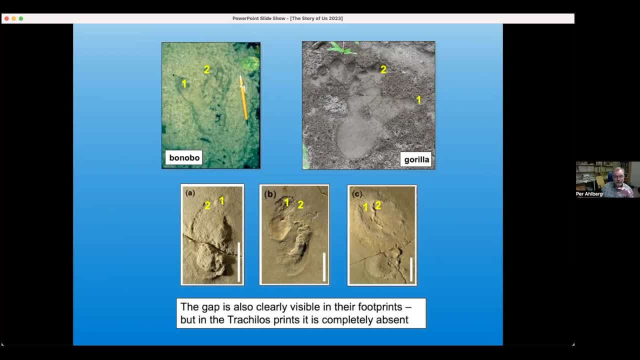 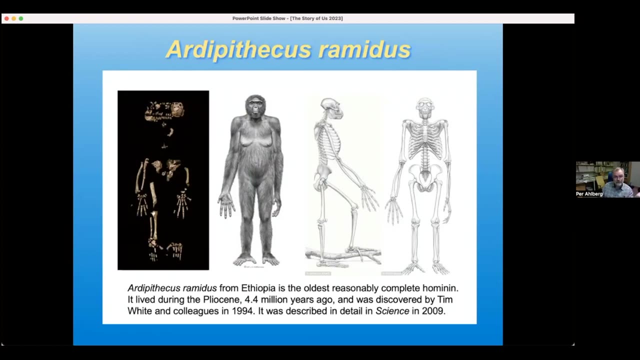 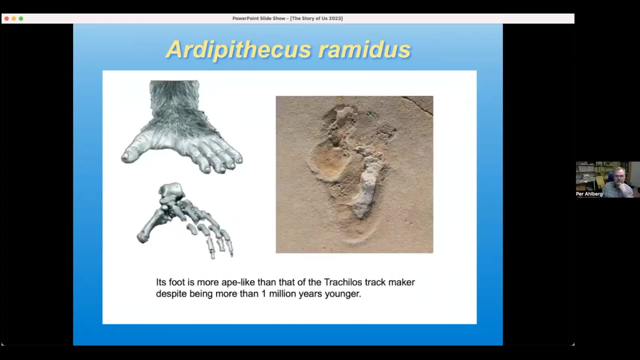 prints, which is uh um, approximately coeval with aurorin in in kenya. what's also really interesting is that if you then look at our at ardy pythicus um a little bit younger than four and a bit million years, lovely material, quite extensive, very nice foot. foot looks like that. so 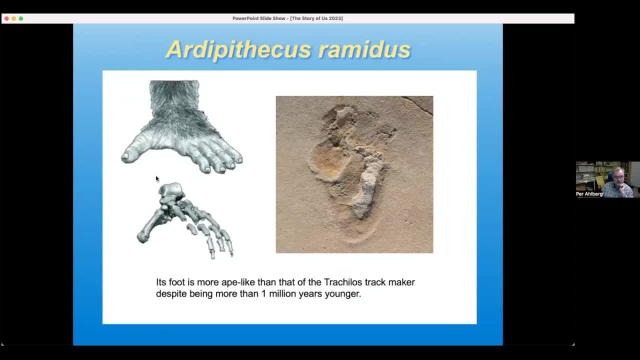 assuming that all the bits of ardy actually go together and this really really is the foot that goes to the rest of the skeleton. it's clearly an eight foot and, um, if, if this is a hominin, it must be further down in the human stem group than this, that's. 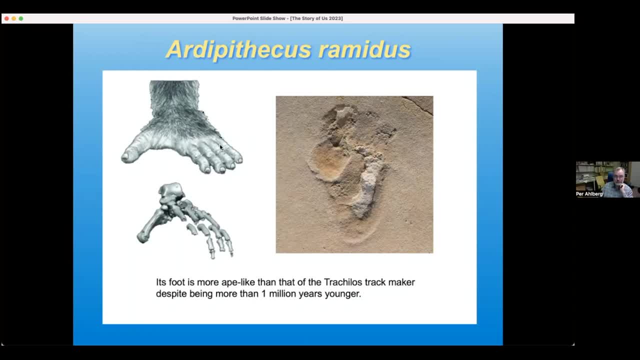 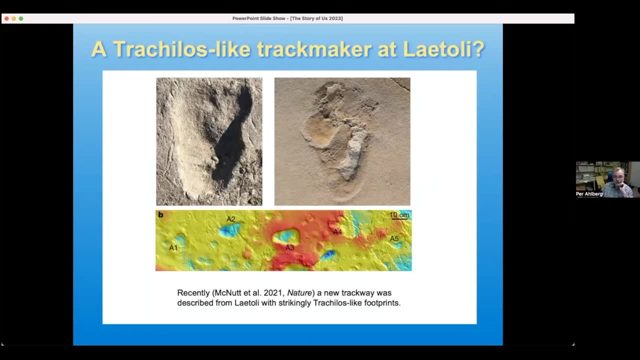 because you know, we have derived characters here that are simply not present in this thing. other really interesting thing that happened a couple of years ago now, which, again, i'm sure many, many viewers will be aware of, is the description of a new trackway from lay totally. 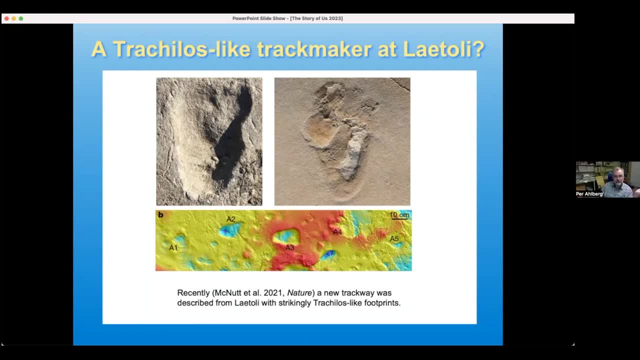 well, actually an old trackway from latolia had been discovered in the 1970s, but but properly studied and described two years ago in nature by mcnutt hotel. uh, with a foot morphology quite different to the previously known, late holy prince, because the classic late holy prince 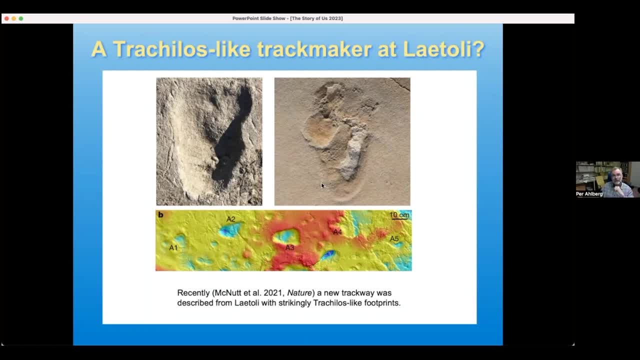 are. i don't have an image or one here, but they're obviously more human-like than the the tracheolus prints in that they are much longer and narrower, with more of a heel on them, but not these like that. it's an absolutely remarkable and remarkable work of art, and i would just like to say thank you. 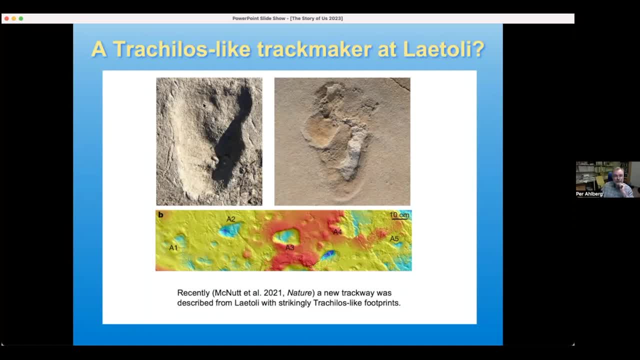 remarkable match and it seems to me, in the first instance, absolutely clear: this new, late holy prince can't be made by the same animal as the old, late holy prince. i mean, forget it, you know, look um, granted, these are a bit blurry and all they're made in volcanic ash, but but nevertheless. 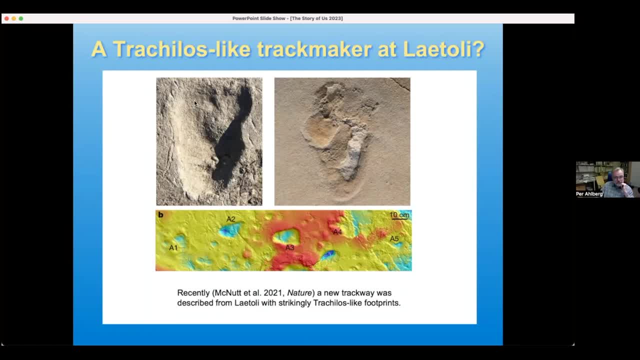 what this does suggest, to my mind, is that you have, at this time point- and this is what three point, something million years in east africa, somebody walking around with feet that are really very similar to those of dracula's track maker. so so, so you know, there, in essence, it's the. 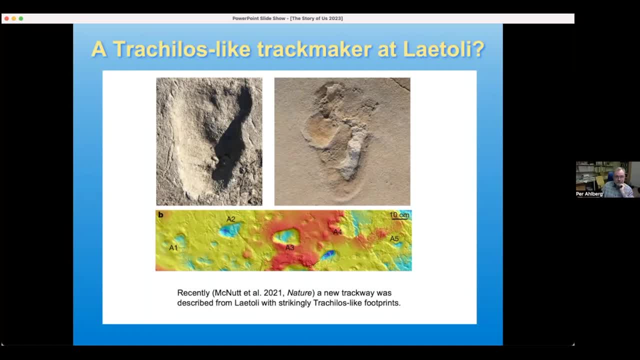 story of this um, it's, um, it's not being received with universal joy in the paleoanthropological community. i think it's fair to say, but i do believe it's. firstly, i believe it holds up. i mean, obviously i believe it holds up, but i wouldn't be sitting here, um. but i also think 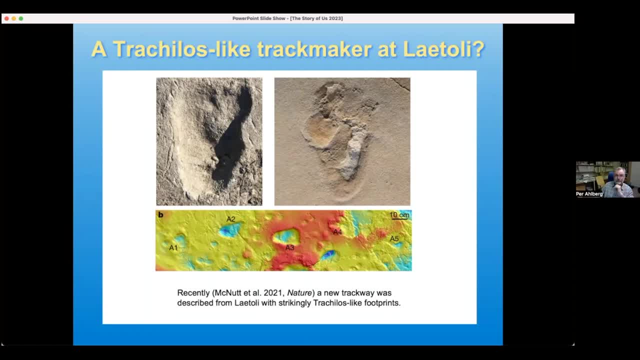 that it is potentially really informative about a very early phase of the evolution of human bipedality. well, first of all, i thank you for putting this little presentation together, because it's brought some attention to my eyes that i did not previously give credit to, because i was one of those people. 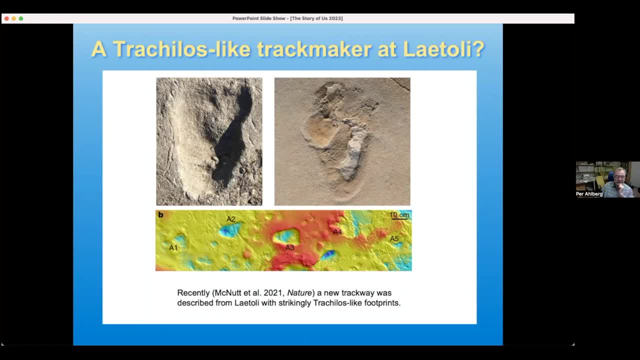 who? oh, the greek footprints, you know, yeah, whatever, but um, especially looking at this image which, right after this paper was published by mcnutt, at all, um, i had her on the show and she was talking about her paper and, you know, looking at that specific footprint, which i believe was from track a, um, they did they, uh, the researchers. 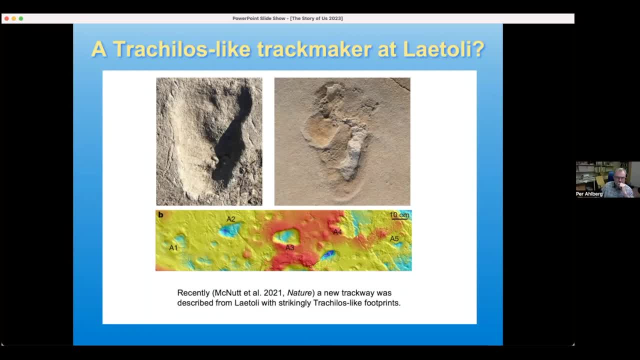 on the paper. agreed for sure. it definitely was not the same creature that made the rest of the print. yeah, i think that's absolutely clear. i mean i i know those opinions diverge about that in the community. i've had some discussions with some people who are wanting. 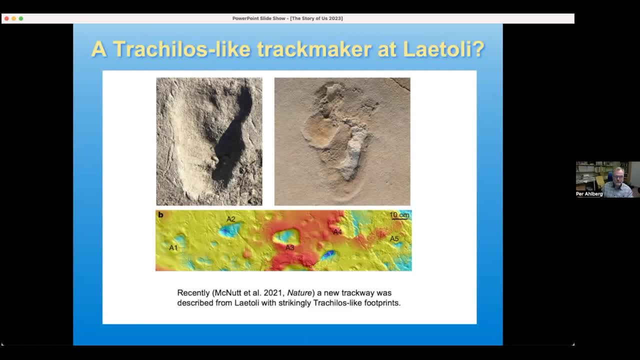 to argue that you know all the late holy tracks are made by the same taxon and that is all. just you know preservational differences. but i think this is nonsense. i mean, you know i i cannot see how the feet that made the classic late holy tracks would also make those. it just kind of 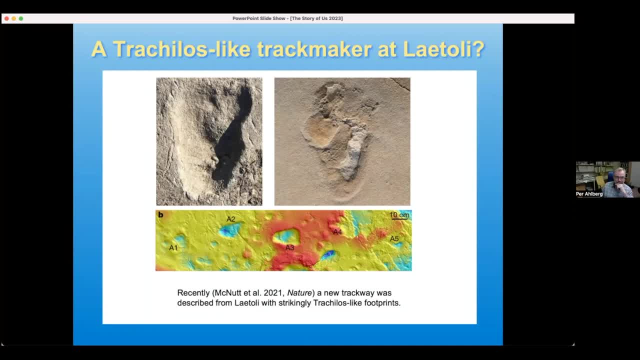 you know, right, they just they just look extremely different and the scans and the, the analyses that her team did are not the same as the ones that she did, and i think that's something that i think we have to think about, and i think that this is very much a. 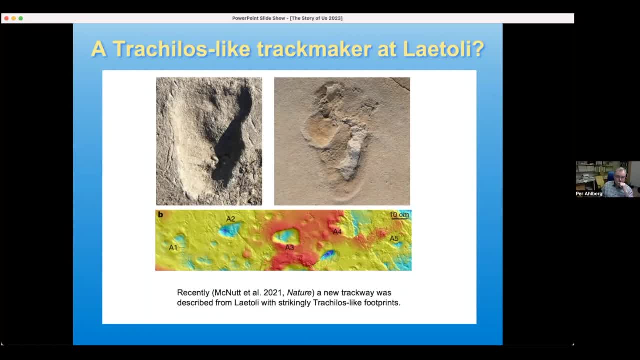 criticism of the fabric because, um, i think this issue of the senate is so tough and so bad. also because, um, i think it's better to stand up and say: you know what we did? something definitely is bad. it's not something that we should, as a community, would do and not. 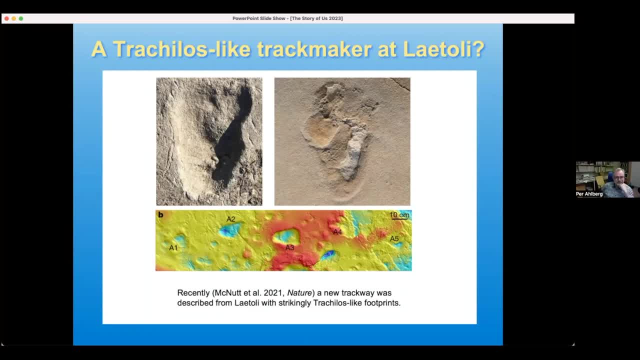 get too involved in this kind of thing and i think, um, i think that's really important that people get involved in this kind of thing, and i think we all have things that we need to be able to do and be able to think out of that system and, you know, that's the thing that we can't儿. 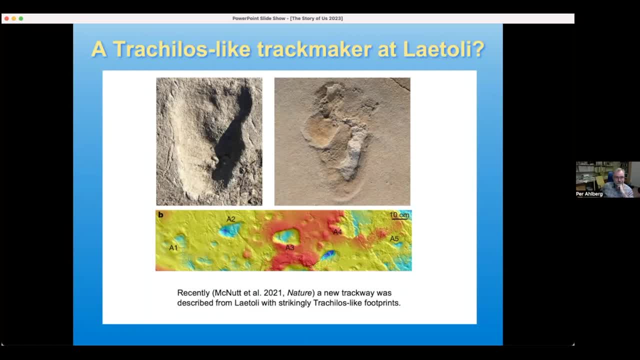 i think everything really shows that. i think that there was a different hominid out there which pretty much, yeah, and they're looking across and they're standing there is something else. yeah, it could have looked back and they could have made eye contact. and these two different. 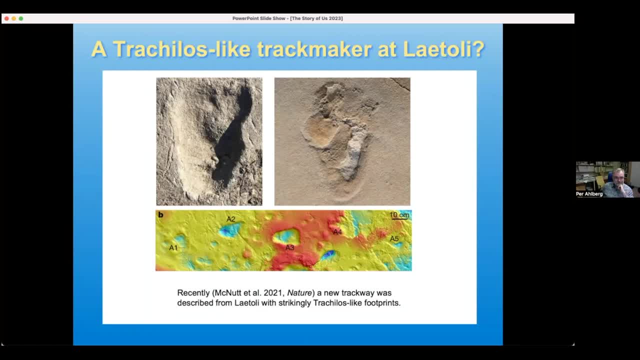 hominids, hominins, that you know, because what 20 years ago people were saying, hominins couldn't live linearly and not linearly, they couldn't live bilinearly- um, yeah, but i mean, i think, i feel that, firstly, i i absolutely agree what you're saying there and i also think that there's 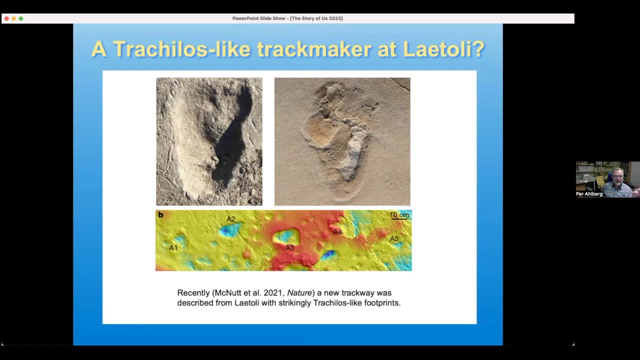 there's a there's another point about this that one needs to think about. if there's one thing that sometimes troubles me a little about the paleoanthropological research world as such, is the fact that there's a certain sense that people easily lose sight of the fact, especially 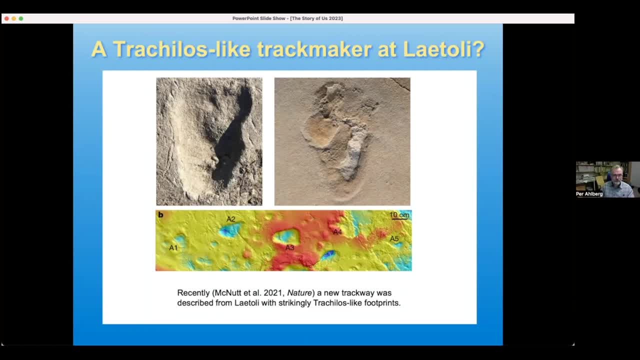 when we're dealing with these very early animals, with myosin and pliocene. that, look guys, we're talking about neogene mammal evolution and neogene mammal biogeography. nothing else- and i mean saying that you couldn't have two hominins living side by side- is about 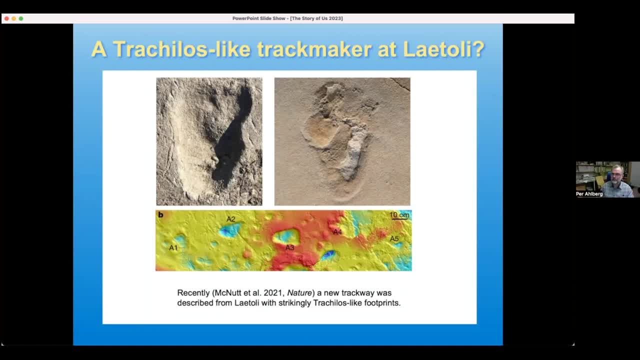 as daft as saying you couldn't have mule deer and white-tailed deer living side by side, which you can. you know why the heck, wouldn't you? um? and it's now, yeah, sorry, sorry, um, for my audience sake and for my sake as well. neogene- i don't think i've heard that term before. 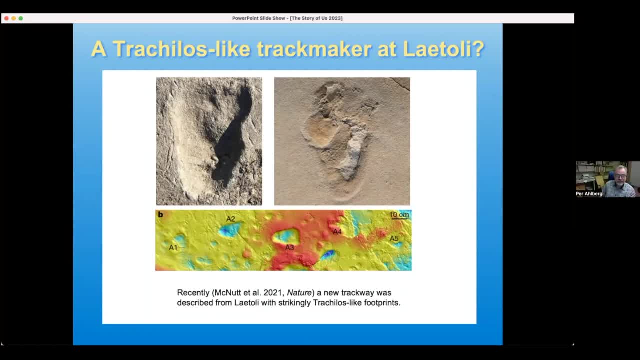 sorry, i thought i might be familiar. no worries, i'll explain. it's simply the later part of the what we'd otherwise call the tertiary. so the paleo gene, that would be like paleocene, eocene, oligocene, um so long ago, and kind of weird animals, and the neogene that's um that's. 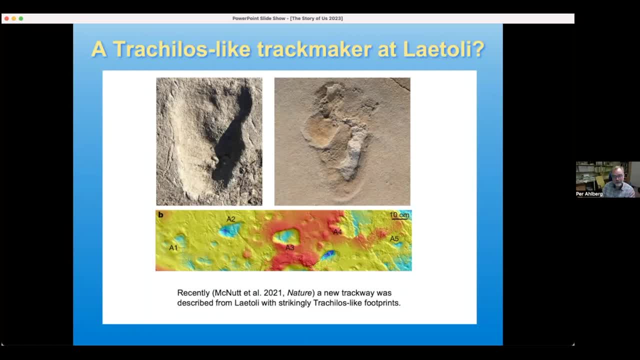 more recent times, so that that's myosin pliocene um pleistocene, but in other words, i mean, you know the it's it's not all that long ago, it's not all that long ago. it's not all that long ago. but the key thing, what i'm sort of getting at here, is that we're dealing here with a really 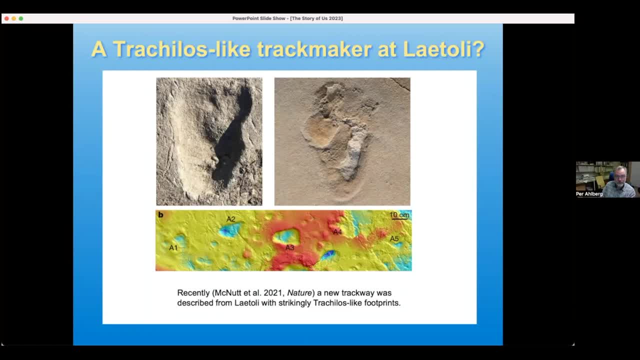 early part of the of the human lineage and while if you're looking at, i mean obviously modern humans, but let's say, if you're looking at what you want, neanderthals. of course you know, yes, yes, we're animals, they were animals, but we're a bit different as well, and we we can be assumed to have been. 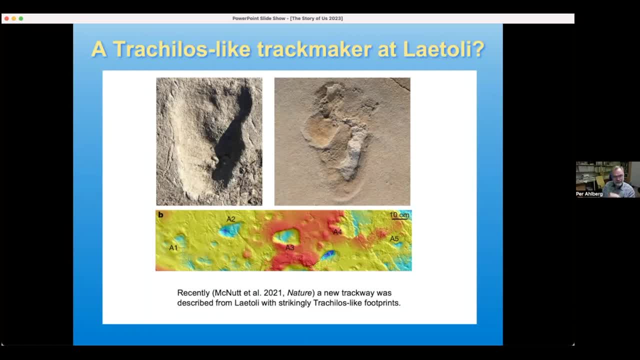 doing really rather different things. but these guys, you know, two, three, four million years ago, i mean, they were animals full stop by any reasonable measure, like chimpanzees walking on their back legs, and there's no reason particularly to think that they would be, that they would be, that they would be different in the sort of 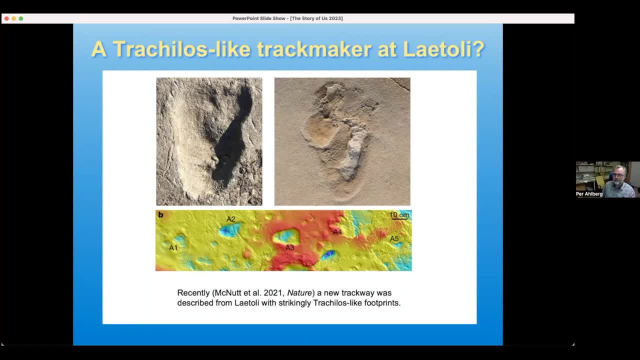 general parameters of their existence um than other mammals, if you see what i mean. but the problem is, of course we tend to look at them from the vantage point of us, as you say. it's the story of us, right, and so one will be inclined to look at them and and mythologize, if you see what i mean. 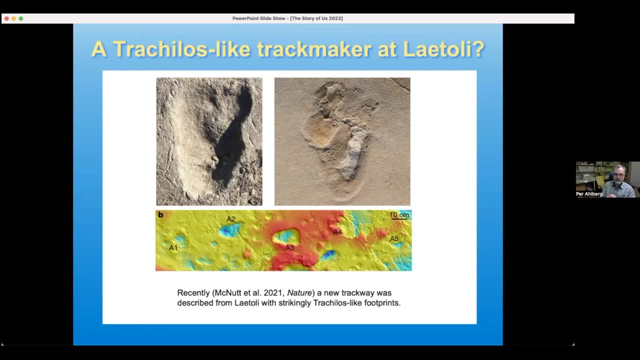 it's. it's very easy to think of it as some kind of heroic lineage leading up to ourselves where perhaps a more generically kind of mammal biology perspective would be more helpful. i think a little bit of that is still people looking for the missing link. yeah, i think there's. 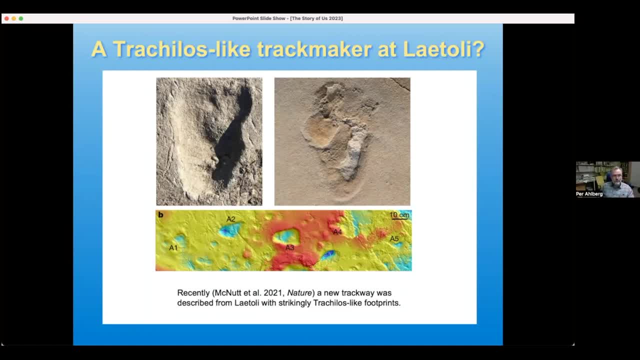 a measure of that going on and, to be honest, i think this is this is where we have a little bit of an issue with, with, with the business, with the, with the biogeography. i think it's a bit of an issue as well. i want to say a few words about that, if i can, because this is one of those things which 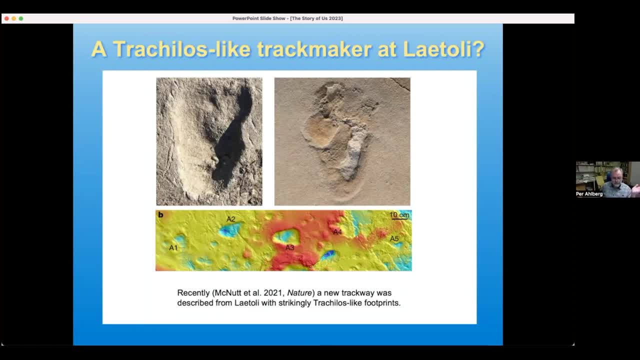 we've been kind of bumping up against. um, the very first thing to say, just to sort of set the scene here, is that while these footprints are from the island of crete, this wasn't an island back then. um, we're looking at a? um the southernmost little peninsula of the balkans. basically, it was attached. 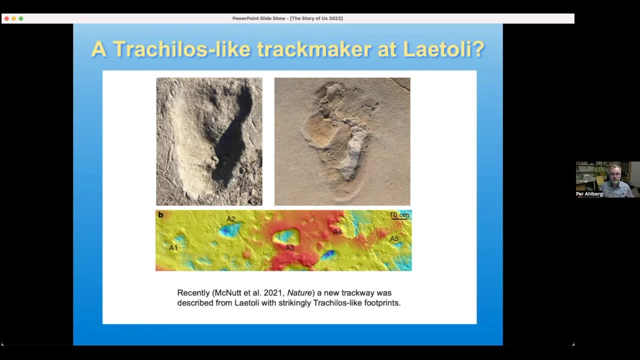 to the mainland and you have, you know, both in the sort of trackway fauna from crete and, from a slightly older body, fossil fauna. so this is, like you know, this is the southeastern european mainland, um, nevertheless, um, quite a few people have argued that this isn't plausible because it's a biogeographically outrageous. 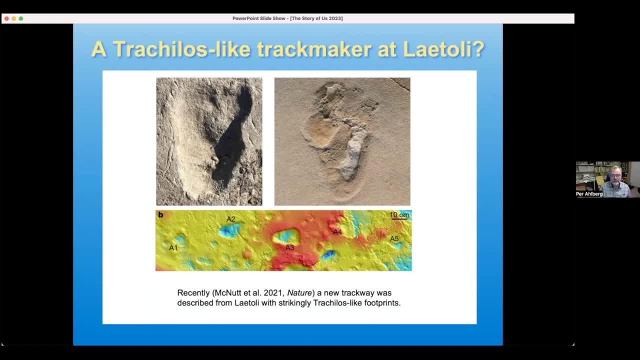 hypothesis and i think it's a complete nonsense. i can see what such a hypothesis were if i were to come trotting along saying i've got my seen hominins from north america. that would be outrageous, because it would be. you know, you have to imagine a biogeographic spread of these things unimaginably different from from what we sort of. 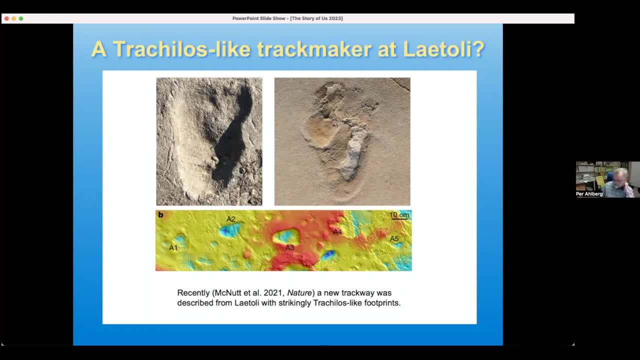 had to hand. but i mean, if you, if you look at, if you look at this general time frame in, in sort of the um, the east, the western part of the old world, if you will, um early in the moose, we have subtropical rainforests extending right up across europe and it's and it's full of apes, um. 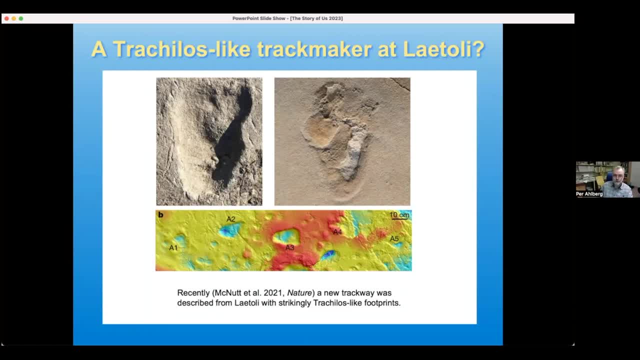 of course we also have- you know it's tropical to subtropical- rainforest- loads of apes in africa. this is not in dispute, but what we tend to think of now as this very kind of sub-saharan african biome where we would find the gorillas and the chimps today, you know, extends all, happily all. 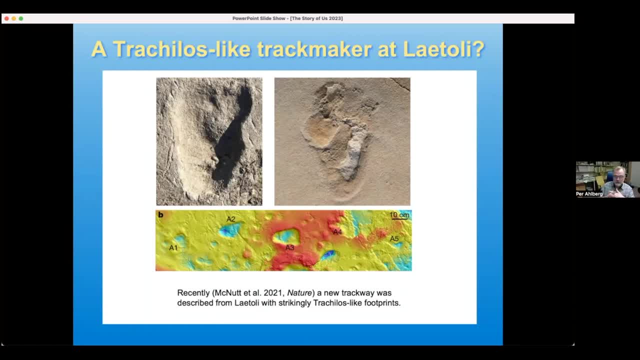 the way up to vienna. um, so it's a very different sort of world and really the balkans isn't desperately far from northeastern africa. uh, if you imagine a context where the environments are still more or less sort of homogenous, i mean, of course, at the time of these, these footprints- 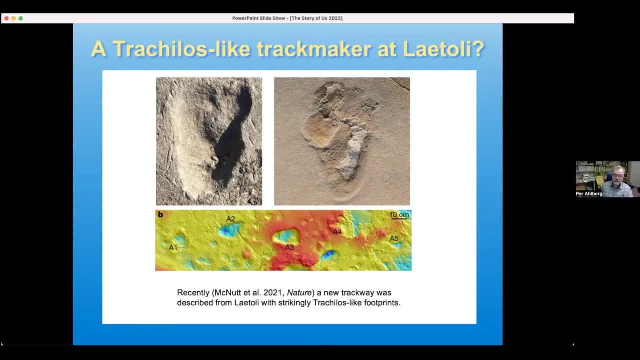 things are starting to change, starting to get drier, it's starting to get colder, the sahara started to develop. so you know, fair and square um, but but the immediately sort of preceding period was one of great homogeneity, from from africa up across europe, and you know that might. 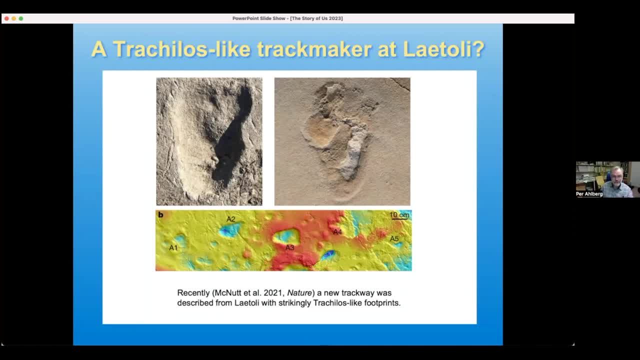 or might not mean that that you'd have to, you know, you'd have to you know, you'd have to, you know, have hominins in in in europe at the time. but the idea that it's somehow inherently implausible or a kind of outrageous hypothesis doesn't really stand up. it isn't a big deal if i was making this. 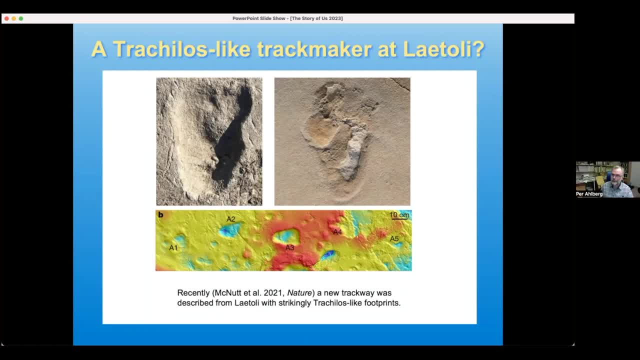 kind of claim about a genus of antelopes or pigs, nobody bat an eyelid. they'd say, well, that's kind of cool, well, that might even be publishable. you know, it'd be so sort of low-key and i think this really comes down to this sort of 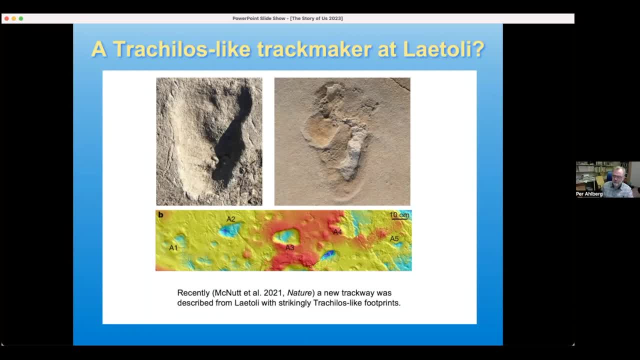 the quest for the, the quest for origins. you want to be able to tell a story and if you land on that story being, the human lineage originates in africa. and of course i should say here: the origin of modern human humans in africa is not a matter of dispute. this is documented and it's just you. 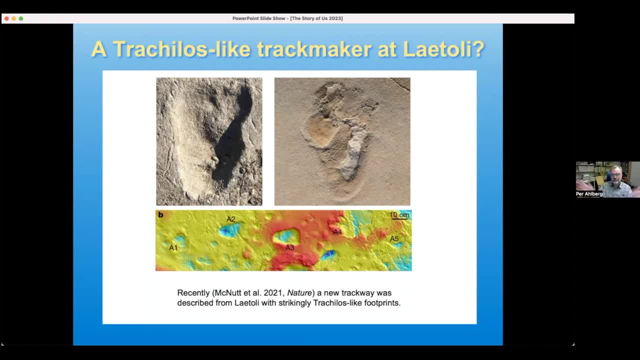 know that that's the the truth of the matter. along them with the kind of spreading out and the kind of interbreeding with neanderthals and all this now familiar story. um, if it's talking about, did the entire human lineage originate in africa? well, it may well have done. 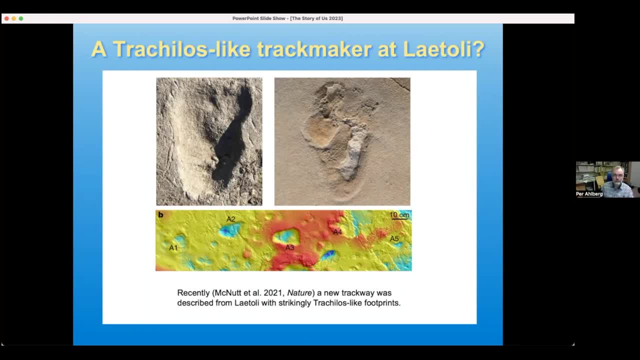 the last common ancestor of humans and chimpanzees may very well have lived in in, you know, central african republic, or it may have lived in bulgaria. there's frankly no way of telling and it's not obvious to me that it matters desperately much, but i think it does come to. 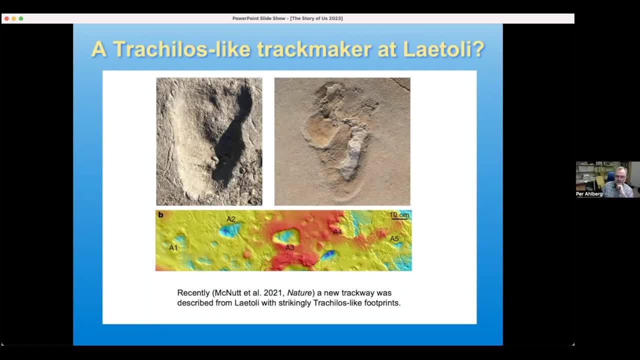 matter to some people and they kind of invest quite a lot of feeling in this in a way that's perhaps problematic for interpreting the science. i think definitely when we're talking any type of science, when bias starts rearing its head on what we want things to be based on. previous 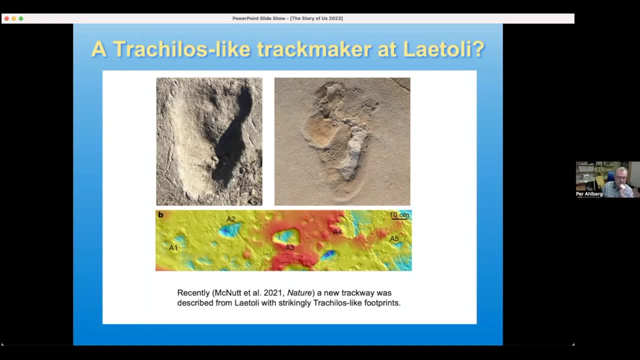 and paleoanthropology is built on what has been proclaimed to be true, so going against it is quite posturing usually. yeah, yeah, i mean. yeah. it's worth remembering, after all, that when the first australopithecine fossils were were presented in the 1930s, this was made with a barrage of hostility. 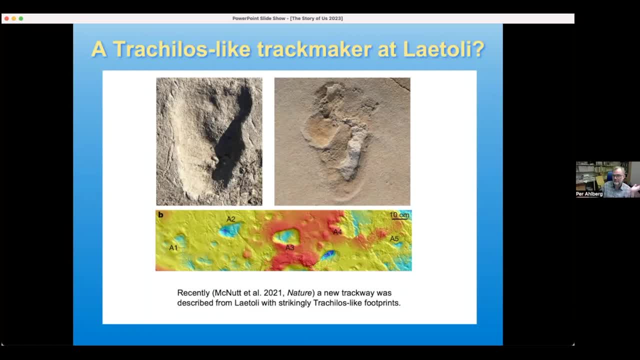 from people that had already decided that humans originated in asia. so you know, there's the there's that my taking is basically this: the biogeography aspect i find mildly interesting, but it isn't a terribly big deal. however, what i do think is really important with the tracolos footprints and 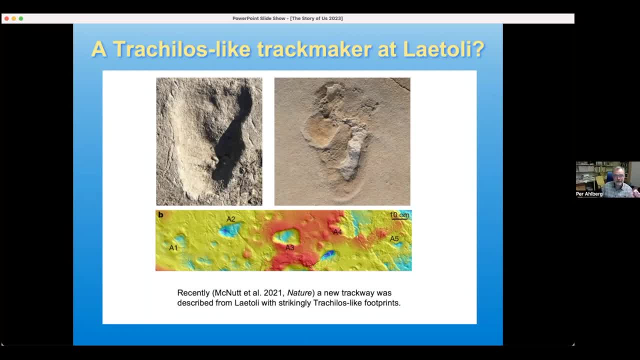 why i am frustrated by the way they are not making much of an impact in the field is that i think they are extremely informative about the early evolution and timing of evolution of bipedality. and that's only gonna, you know, that's only gonna be seen if people actually kind of take 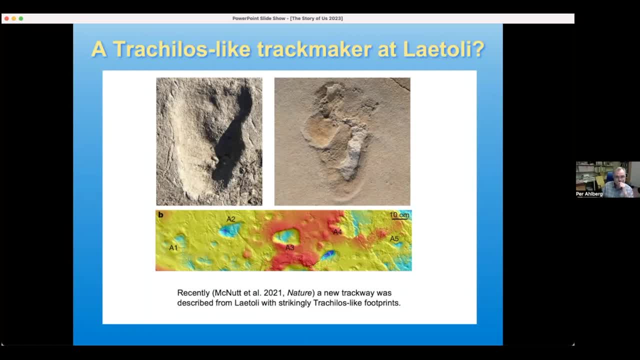 a proper, careful look at them. so how do you think it might reframe what we know about the origins of bipedality? well, i mean, the thing is basically this: um, first of all, just worth noting in terms of we're still looking at this picture of these footprints. is is worth keeping in mind when comparing these two. 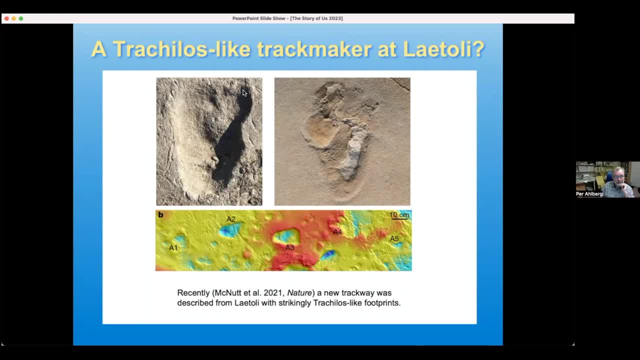 that we have have in one instance a print made in rod soft volcanic ash. the foot has gone quite deep, but there's also quite a lot of loss of detail, whereas here we have a footprint made on what must have been compact wet sand and it's really shallow and some of the toes just sort. 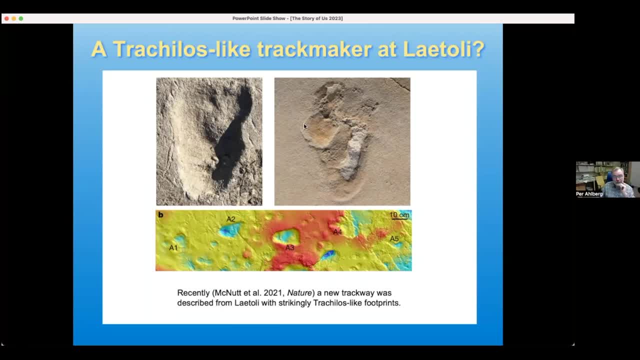 of fade out down here and it's really shallow, and some of the toes just sort of fade out down here, um, but but but. but. the outlines, on the other hand, are very crisp. uh well, i would say, key thing here is that what it shows, assuming then that you know i'm getting. 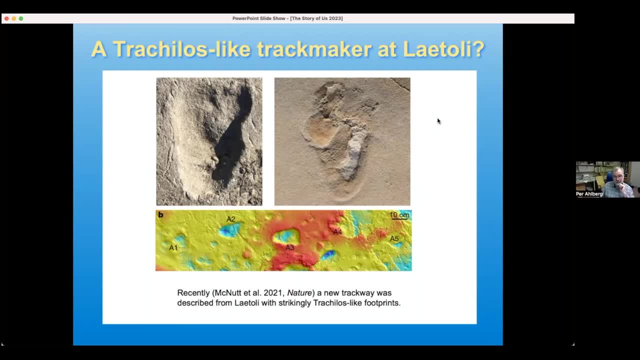 these right and that the dating also holds up, but currently at 6.05 million years um. what it's showing is that at this really very early time in the evolution of the human lineage um, a rather a rather specialized sort of bipedal foot has evolved, the- i mean, of course, this veto. 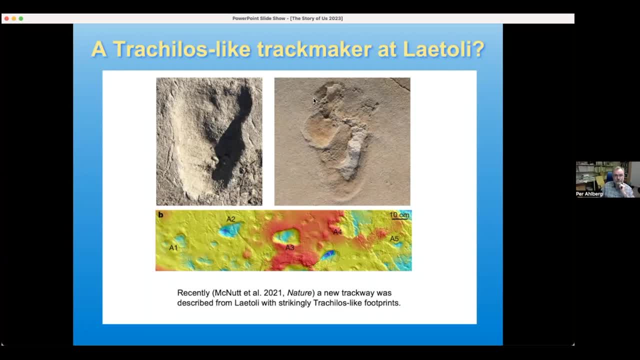 may well be rather more mobile than than in us, and closer, sturdier the footprints may settle that matter, but already what you can see is that it is attached to the distal margin of a coherent soul rather than coming off of the side of the soul, and so it's not its gripping ability will certainly be. 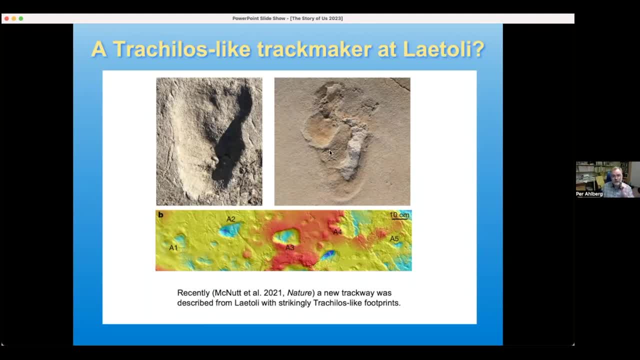 greatly reduced compared to a chimp or gorilla foot. so this animal is downgrading its climbing capability in favor of better bipedality. so that's the first thing it says. second thing it says is that we do this initially by you know, the first thing that happens is that you modify the front. 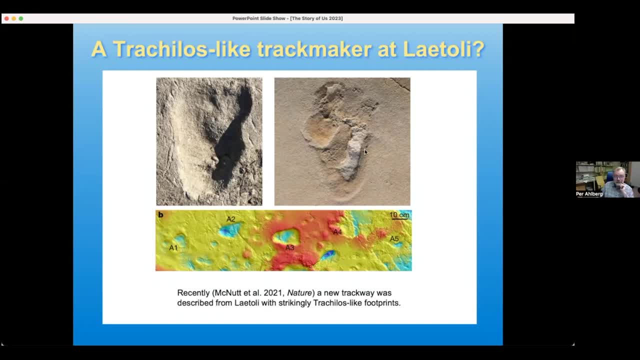 end of the foot, um, the. the lengthening of the soul comes later. we see that in the classic late holy prince. and the swelling out of the bulbous heel and the creation of the arch comes even later. you have that in tracks like illeret, for example, when you're into the genus homo and presumably all of 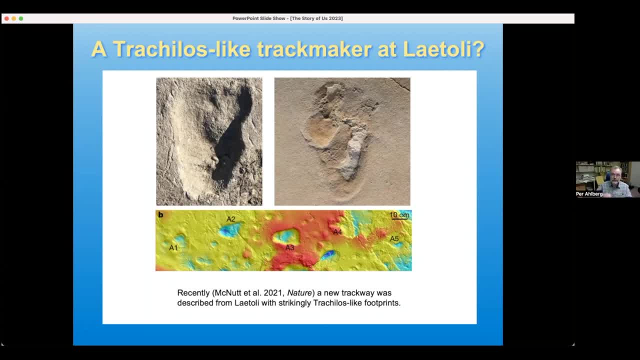 this is related to the transition from a kind of stepping gate. one might imagine perhaps something rather like: you know the way your toddler walks and they've just sort of figured it out and it's sort of foot down like so right, um, from that towards gradually, this sort of rangy rocking. 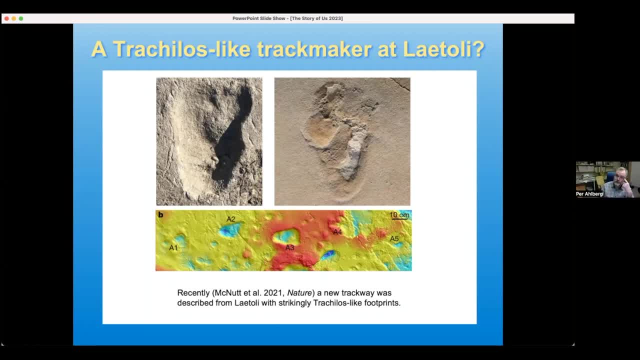 foot striding gate that eventually becomes so characteristic of, of, of uh modern humans and which, presumably, by the time you get to something like in a home or a gaster that's fully developed, because if you look at the- the look at maripotoma boy- you know you've got this sort of ape man head. 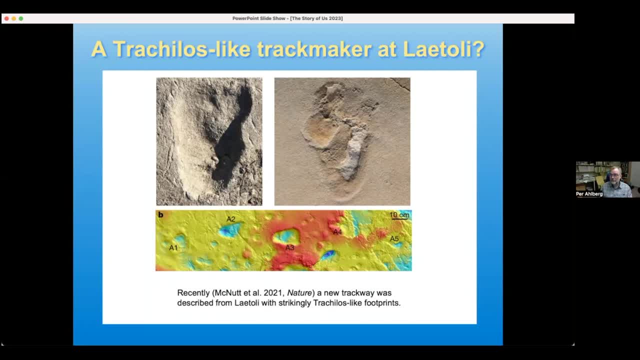 set on top of a what looks like for all the world, like an entirely modern body with great long legs and everything. um, so you, you can begin to break down the transformation of the foot into steps. well, i mean, arguably you can already start to do that with the classic late. 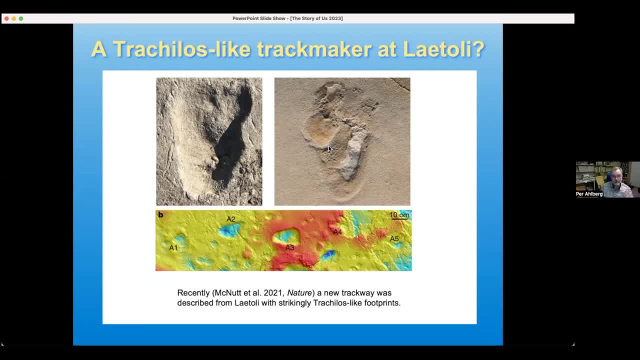 holy prince. but if so, we have another prior step here in the transformation. and finally, as we've already been on to, you can conclude through, i think, considerable surprise that that somebody with this rather archaic foot morphology was still kind of stomping around in east africa. 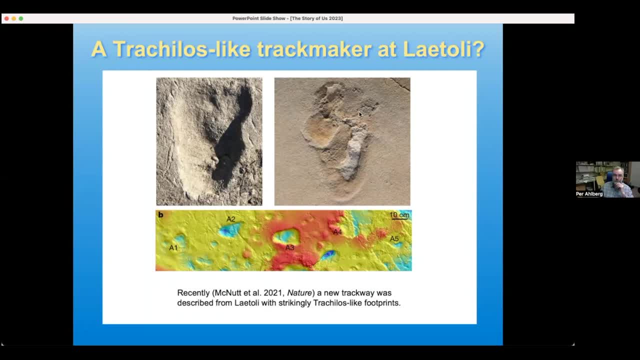 several million years later. so, uh, you know, i think this is this. this is extremely informative, but, uh, but there we are. in order to get kind of, you know, proper value out of these footprints, they first have to be acknowledged for well, actually probably being hominid prince um, and then there's more to do. i mean, this comes from one locality in, in, in. 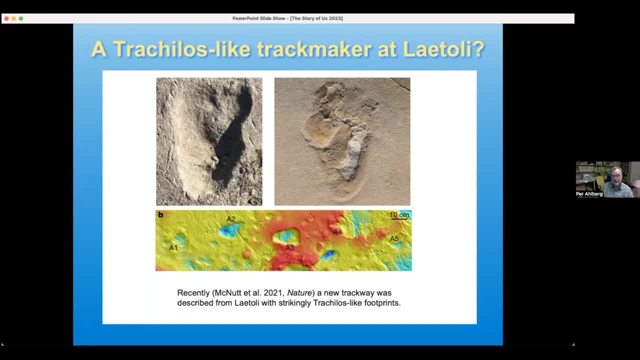 western crete. we need to scour the neighboring landscape for additional footprint, localities and so on, see if we can expand the data set. and for those who don't know or may have missed it, creed is now an island, so some of the surrounding land is now, of course, submerged. so i really yes, indeed. 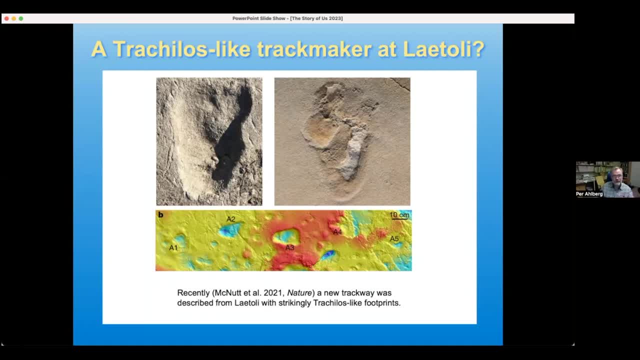 although, you know, crete is still a big place and there's there's a lot of our crop. and, of course, the other point here is that, given given these, there's a there's high likelihood that one might be able to find similar things on the- you know, neighboring bits of the greek mainland. you 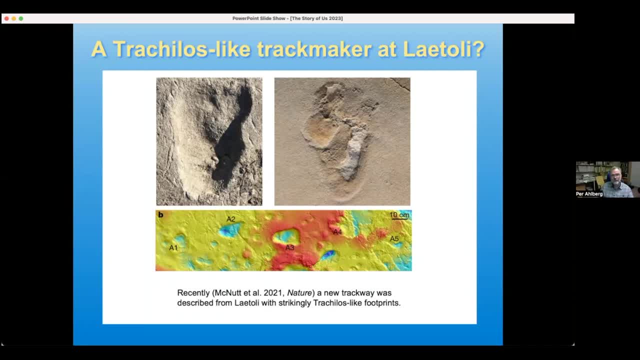 know, the peloponnese, perhaps wherever, and indeed, of course, if you want to think about this as a graphic issue, if we really do have late miocene hominins in the southernmost balkans, um, then realistically they will also have been pressing through anatolia and all down through the levant. 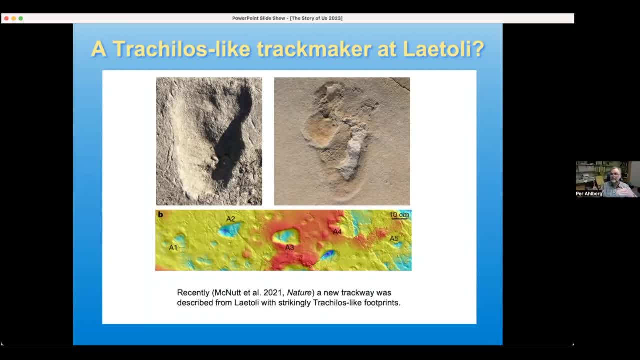 and all down through the sort of, you know, north, northeastern corner of africa, etc. regions which have not really been explored for with this kind of thing in mind at all and where that should be thought about. worth saying, of course, also that i mean you know we have these and then you know you have the great epithecus jaw, and i know that. 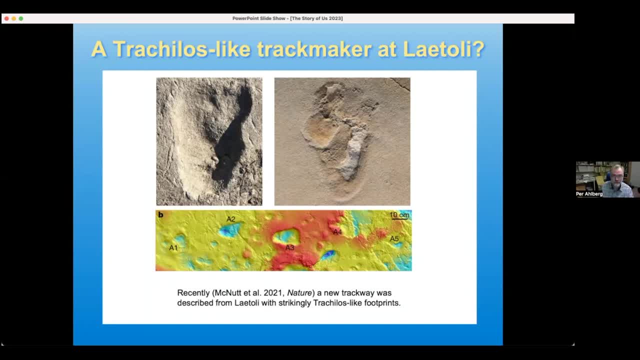 madeline boom and her colleagues are rootling around for more material both in in greece and in bulgaria, and they might find further things there, but all of this is my scene. once we get into plight the pliocene. as far as anybody knows, there are no hominins in europe anymore. 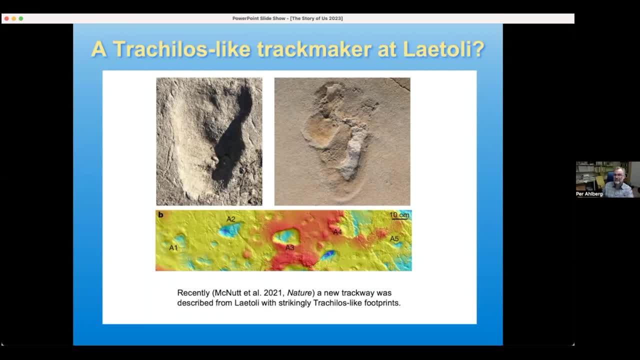 uh, you really are down to this kind of classic australopithecines in africa picture that we're all kind of familiar with, and when hominins then pop up in europe again, you know it's much later. you have things like: you know the money, see homo erectus, whatever, and that's. 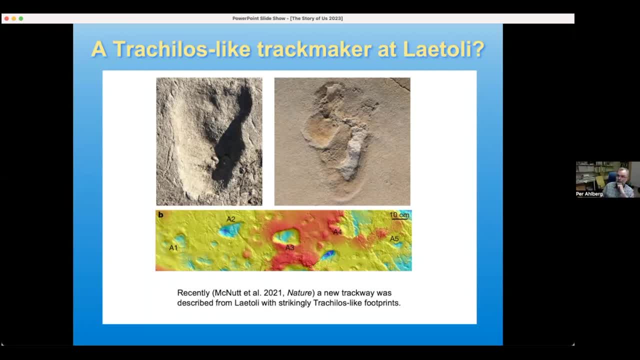 that's clearly a different story and presumably dispersed a lot of africa. so do you think it's possible, since already there's multiple hypotheses on how bipedalism started- that this could have just been an ape like creature that had developed a foot fit for bipedal walking, but then was a dead end? uh, evolutionarily? well, something depends on the. 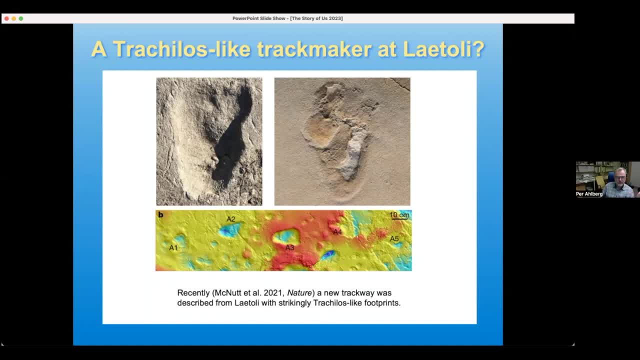 you mean by possible? i mean i mean in a sense, yes, of course it's possible. um, it would be at present impossible to disprove this. in fact, strictly speaking, it would be forever impossible to disprove it. because if you had a complete skeleton of one of these guys and it looked like you know, 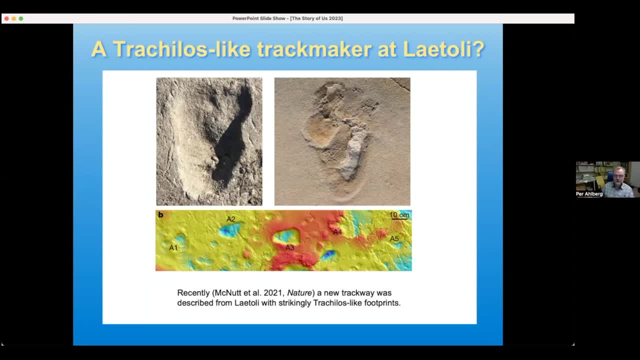 a sort of um beta test version of australopithecus. there would still be no way of there's a philosophical issue here. there would still be no way of proving that that wasn't completely convergent. however, what i would say is: i i think it is unlikely, and my reason for saying that it 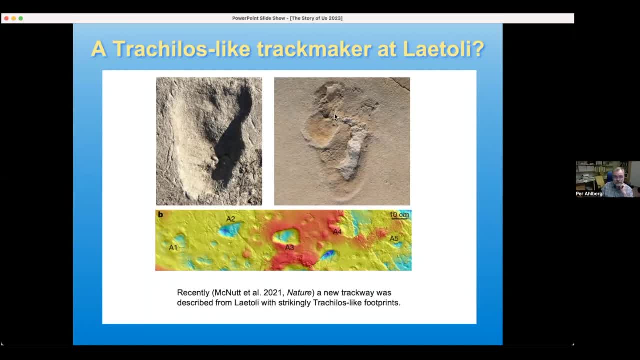 is unlikely is that it shows the specific derived characters for bipedality that we see in, you know, in in undisputed members of the, the human lineage from the sort of late holy tracts up to to modern people. these are the exact same features. now, that's not to. 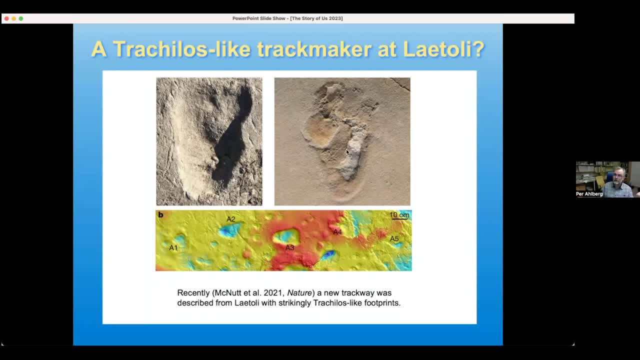 you and you know, and it's not the only way- that you can walk bipedally, um, indeed, in particular if, if oropithecus actually holds up as a bipedal um bipedal um primate, it's a stem group ape. by all accounts, um, it demonstrates that you could be a perfectly good bipedalist with. 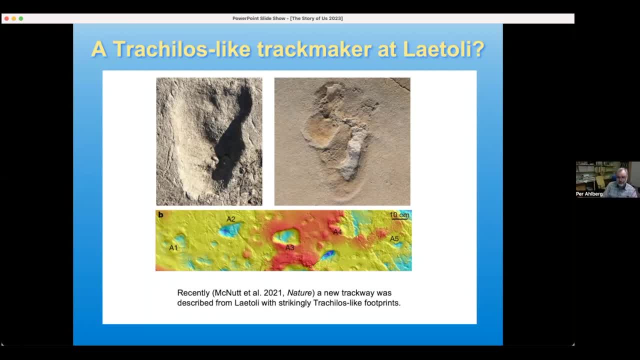 a foot that looks like this. um and again, um, oropithecus would seem to point in the same direction. so, given that it it feels like well it it's, it's kind of a long shot to say that this would be convergent on that, and you'd have to ask yourself: 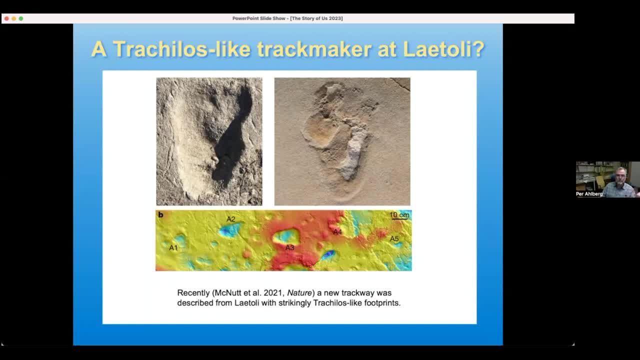 but why would it be? what is, what is the positive evidence to suggest that it would be convergent? um, and i don't really think there is any good positive evidence. so on that sort of paratrooper basis i would reject the convergence. i possibly hypothesis, but but obviously you know. 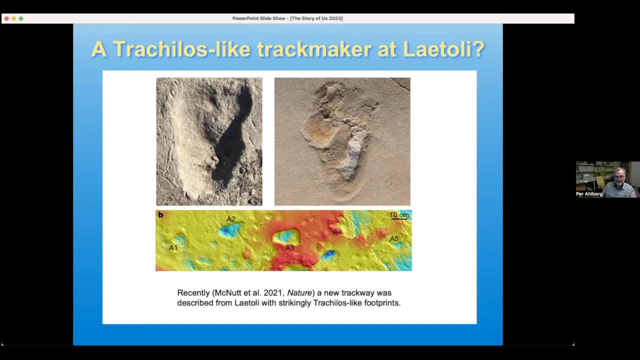 without by that saying it is disproven, because i can't disprove it, but just to say it doesn't really, it doesn't really seem like a fruitful way to go. A better hypothesis would be that this simply is what it looks like And you know once you just look at it. 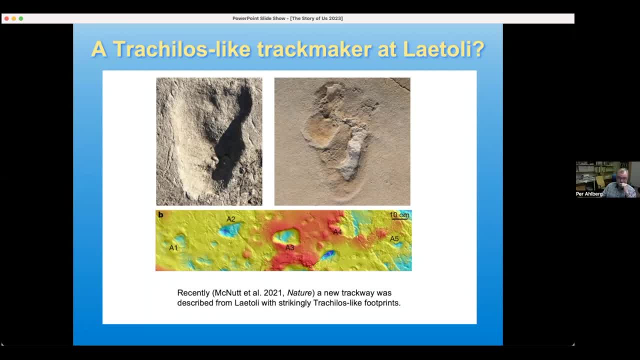 it definitely looks like a human-like footprint, as you were talking about towards the beginning of the presentation, which brings up what I have seen online in a few arguments. Of course, there's the idea that these are natural phenomenon that aren't prints. 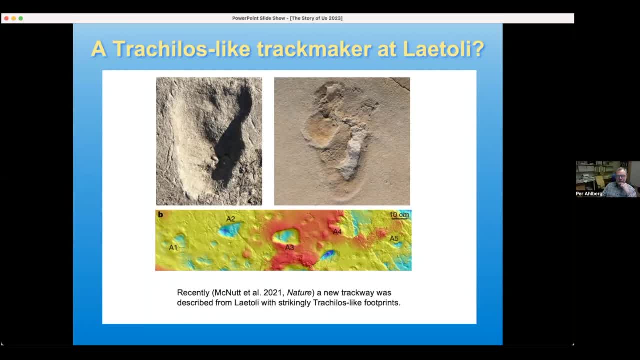 What are your thoughts on that? Yeah well, what can I say? The people who are co-authors on this and all of whom have studied the specimens in the field, between them have more than 400 publications on fossil footprints. 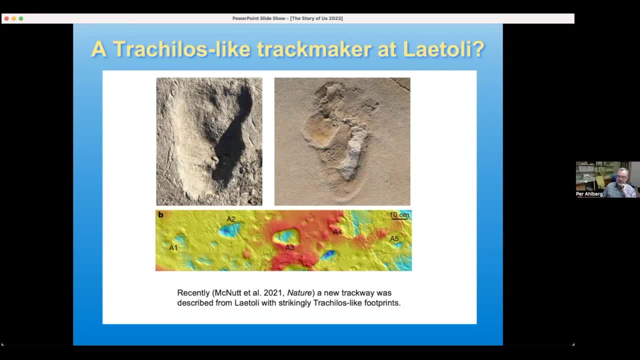 How likely do you think that is It's? you know, this is where things start getting a little bit insulting. but to be more specific than that, if you can see my cursor moving, it's an expulsion rim. It is caused by an object being squashed into the sediment. 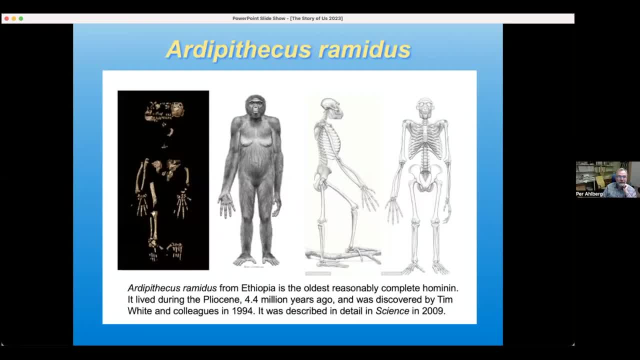 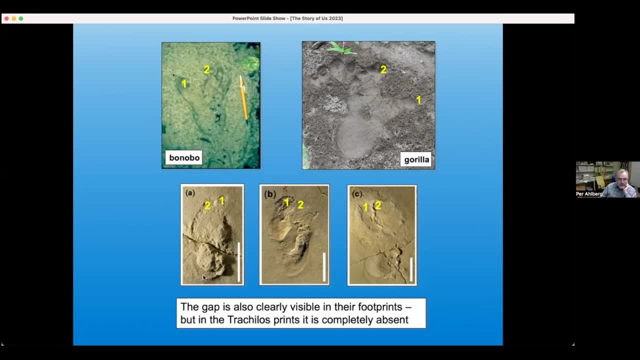 and sediment kind of squishing out. If I go back to the, let's see, yeah, that'll do. It's a bit small, But again here a bold expulsion rim. Let me take the numbers off. You can't see it clearly, but there is in fact. 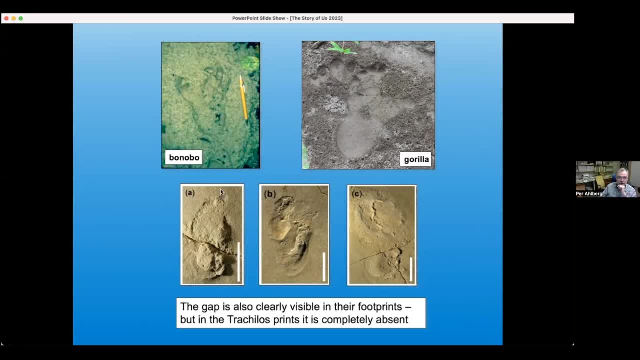 when you have a higher resolution motion for this photo, there's a little toenail drag up here, and here you have the entire run of toes, A critique to say that these are just natural phenomena, that these aren't footprints at all. 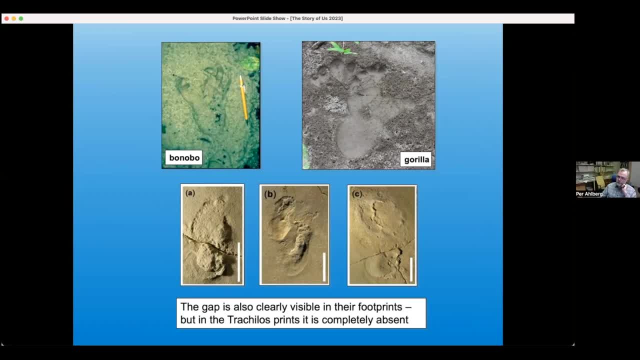 is not a plausible critique and, frankly, not one that deserves a response from people who are specialists in this field. Look, I generally work on body photographs and I'm not a specialist in the field of fossils. And if I rocked up with, you know, a fossil skull? 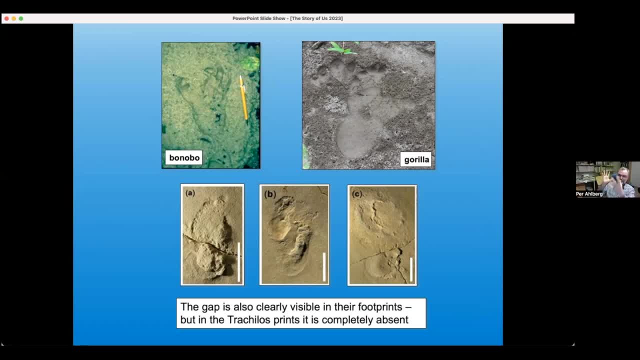 or whatever, it might be a hominid or anything else- and I said I think this is, you know, a skull of this particular animal. a critic saying, well, yeah, all right, but I think it might actually be this other taxon. 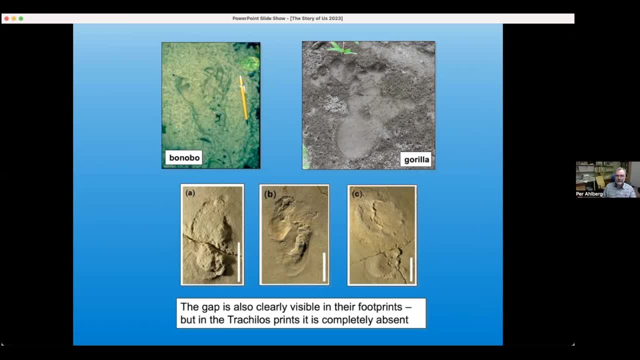 would be reasonable enough. A critic saying I think that's just a rock with two holes in it that look like eyes would not be a reasonable criticism, So that one I think we can dismiss. What does puzzle me with this is that it's not just a rock with two holes in it. 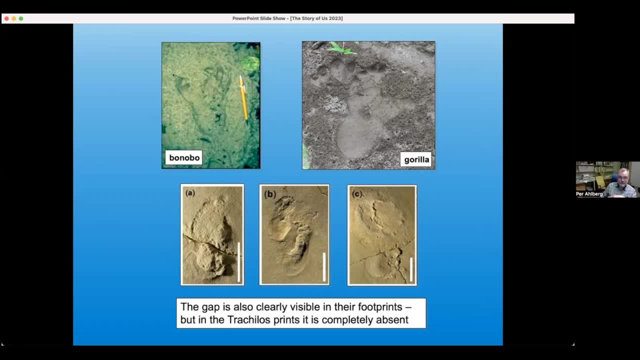 that look like eyes. It does puzzle me with some of the criticism that I have seen. I mean and notably in the published criticism by Sarmiento and Meldrum and in fact, with the correspondence I had with Sarmiento about this. 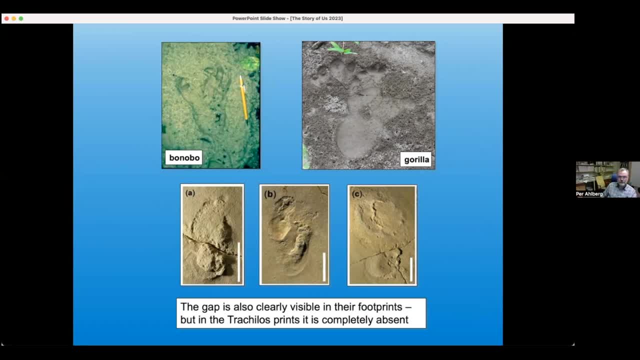 was that they're saying: well, look, it's just an ape foot, No, it's bloody. not. Look at this thing. I mean, I actually had Sarmiento saying to me that, well, bonobos have footprints like that. 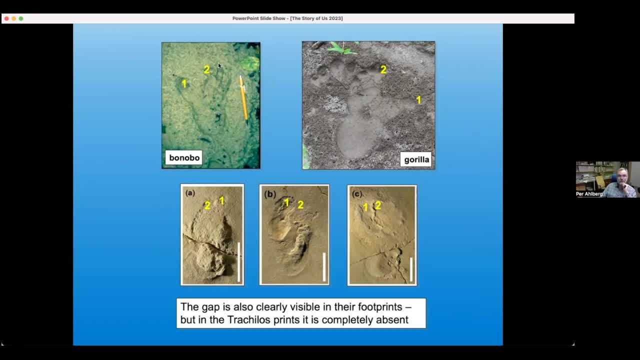 And I sent him- I think it was in fact this very photo- with you know, this huge gap between digits one and two and this completely different look. Yeah, at that point the correspondence ended. He didn't reply to me again. 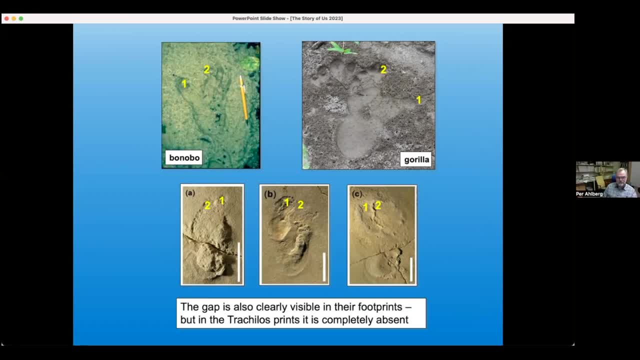 You know I mean, what can I say? I'm not wanting to make people look bad, but this is stuff that I have had to deal with and it's, frankly, frustrating. I'm yeah, yeah, You know people. 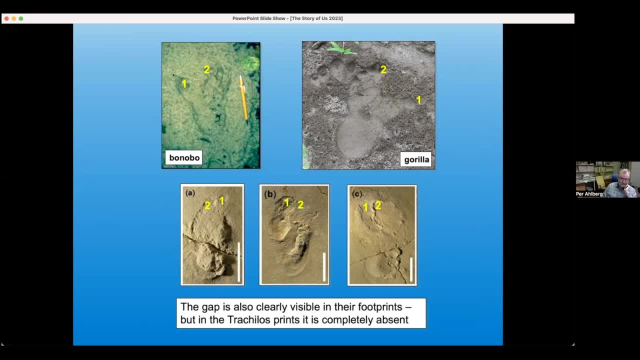 I think, as I mentioned earlier, once they're set in their ways, it's so hard to shake them out of things that the idea that I think is lost in modern day science is: you have to keep an open mind As soon as you close. 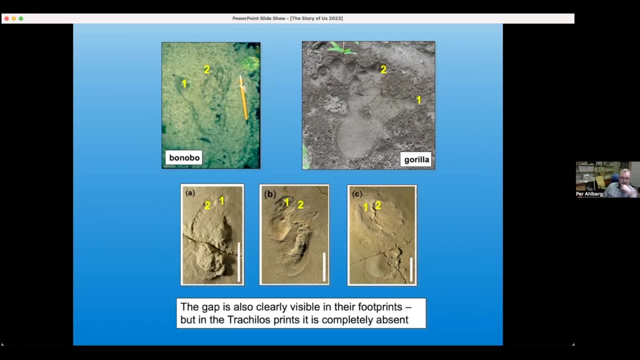 as soon as you close your mind to what's possible, you're not doing science anymore. No, I think that's right. I just want to flag something, by the way. It might be of interest to people who are watching this We have. I mean, obviously you don't have photos of these. 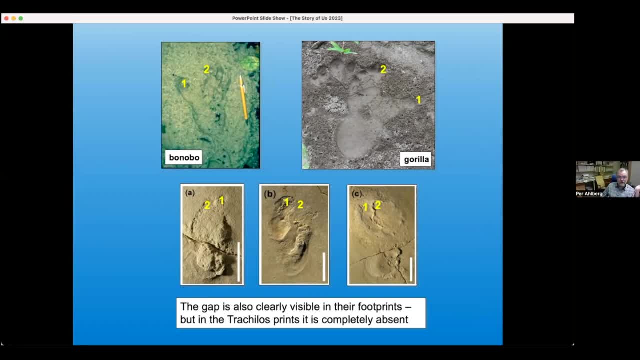 We have a complete set of 3D optical scopes and optical scans of the footprints available as STL files. So anybody who actually, kind of you know, works in this business and would be interested in having a little bit more of a look at them. 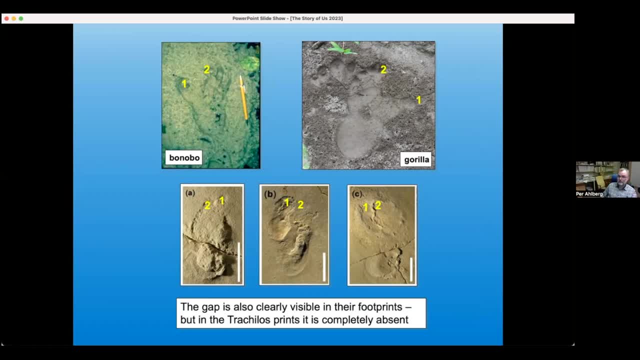 they are available. I mean feel free to contact me and such stuff can be forwarded. You know that, then, means that you can- you can wiggle them about in 3D and you know you can render them in a rendering software like Blender, for example. 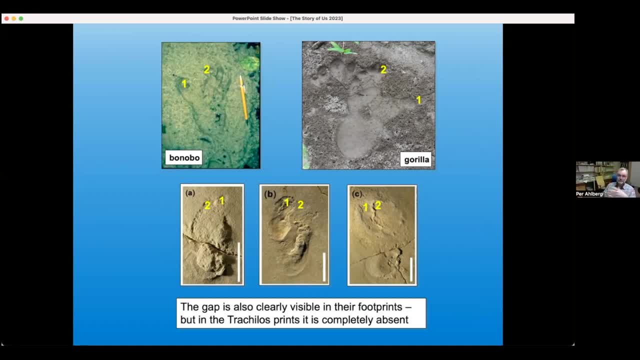 and light them however you want to light them, or a good picture of what these things are actually like. And of course there are, you know, higher resolution photos than the published stuff and whatever too. Right, I'll definitely put the contact info. 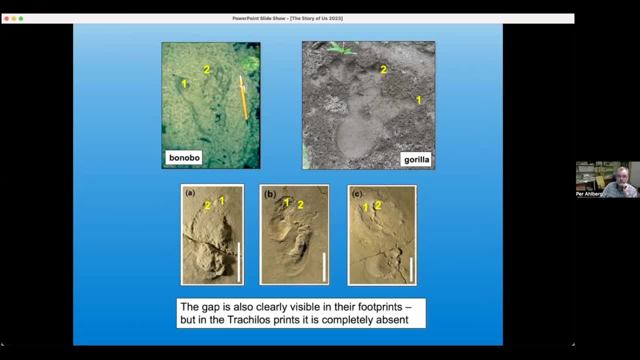 that you give me on there so people can contact you for that, because I think that's a great resource. Yeah, no problem, Just put my email address on and then you know we can sort that out. We don't currently have these, like you know. 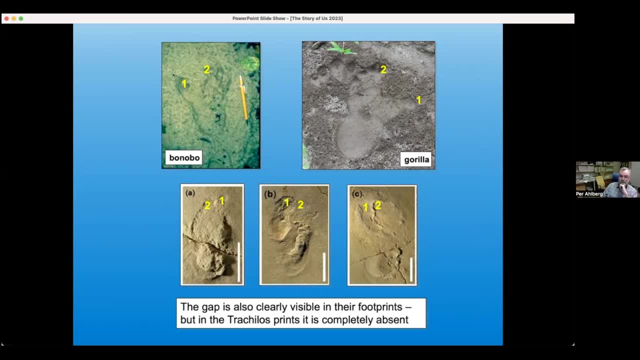 on the server or something, but I can easily arrange for them to be sent over for anyone who's interested. Awesome, Awesome. I think people would really appreciate that. So I think, unless there's anything else you want to add, this has been a great episode. 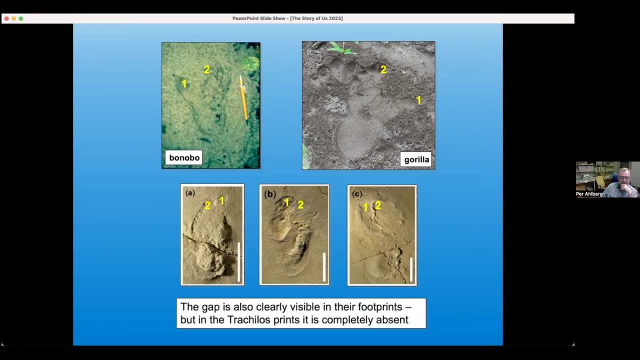 on these footprints from Crete and what they mean for the origins of bipedality. what we're looking at for the older out-of-Africa theory, not the what we're, you know, the recent out-of-Africa theory. 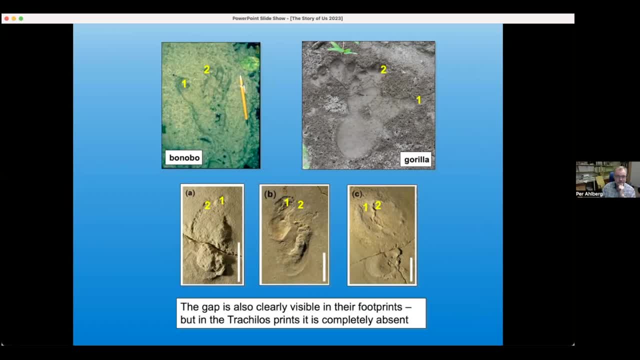 because, as you said, that is solid, We are. we know that's what happened. One question I guess I have is: did this creature, do you think, come south from Europe or come up north from Africa originally and then go back down south? 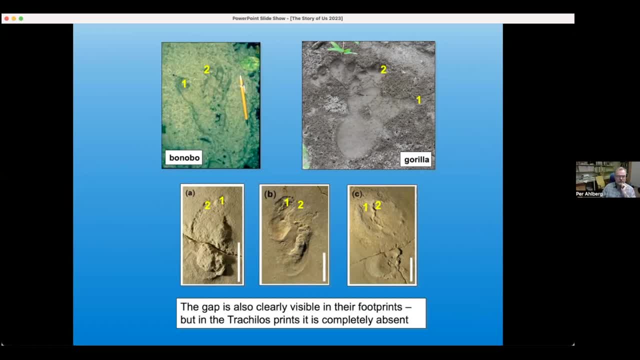 That would be. it's a really interesting question and a difficult one to answer. I mean, the short answer is that at the moment, we don't have enough information to say. What is, of course, very interesting is that, you know, this is contemporary with Auroran. 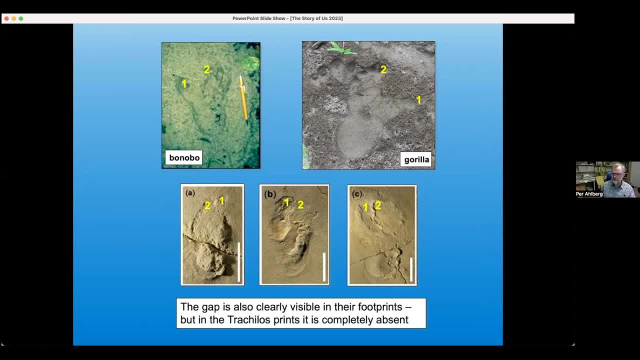 You know, for all we know, this could be Auroran, This could be the footprints of Auroran. You know, it's not impossible, but we have no way of pinning that down. However there is, I mean obviously. 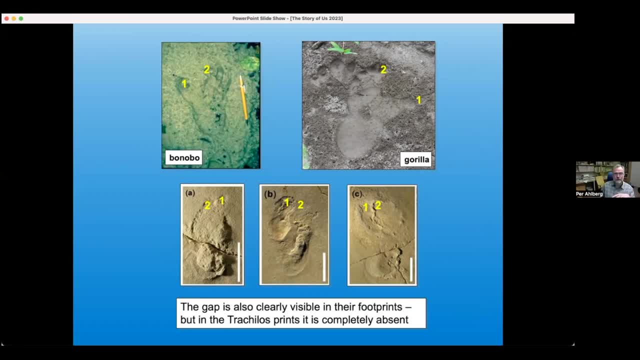 there are people who have their own particular hobby horses about where they might like to see the origin of humans. There's obviously an out-of-Africa gang. There is also an out-of-Europe gang, And I tend to sort of stay away from that entire discussion. 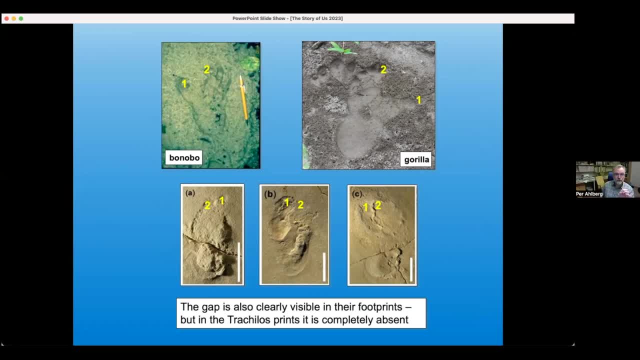 There is perhaps one piece of data that could point to a northern origin, and it's this that I think we're all agreed that the emergence of hominin bipedality and terrestriality is linked to an environmental shift, drying conditions and the breakup. 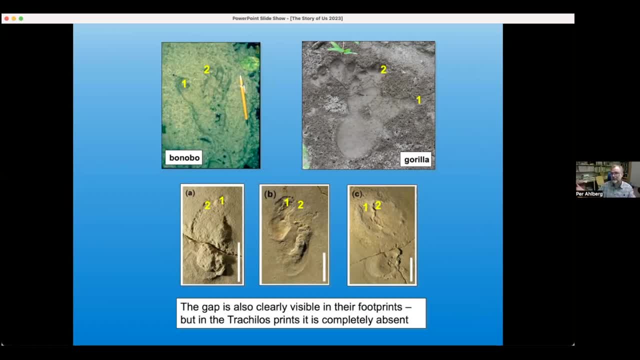 of previously closed forest into sort of open gallery forest and savannah and all of that right. This is uncontroversial And we are again familiar with this as something that is happening, broadly speaking, in the run-up to the ice age. 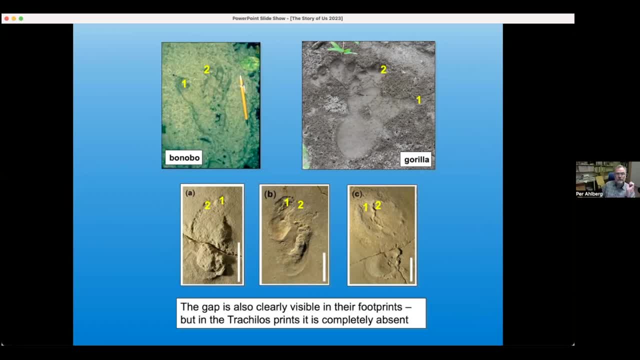 However, what not that many people perhaps are aware of is that this is a process that starts in the north. It actually kicks in in Europe rather earlier than in East Africa. It's already in full swing in Europe during the late Miocene, And this is where we see the kind of you know? 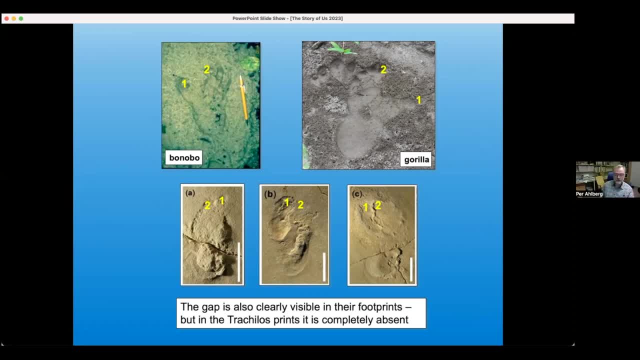 ape fauna of Europe really dwindling rapidly. like you know, early or mid-Miocene There's loads of apes in Europe, very high diversity, And then they sort of dwindle down and dwindle down, And so of course there's a lot of research. 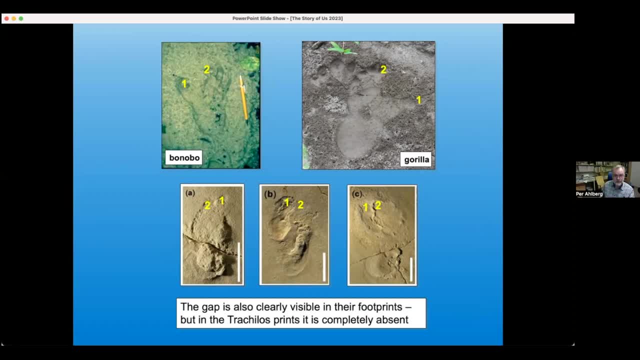 going on about this, And of course one could make the argument that perhaps then the move onto the savannah actually happens, you know, somewhere in this northern range, when the savannah environment first kicks in, And maybe these forms then track the savannah. 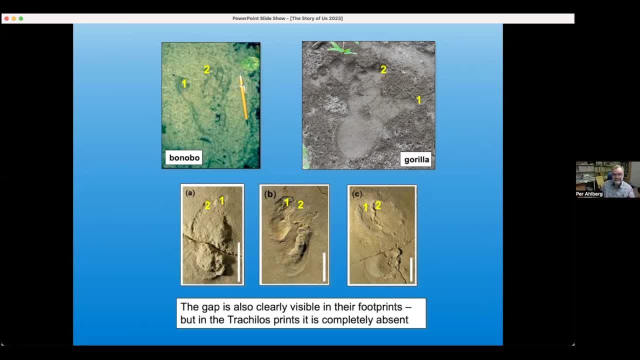 environment down into Africa. But you know that's, It's an intriguing thought but by no means conclusive. And I'm entirely open to you. know an African location for the human-chimp split? At the moment I really don't think we can tell. 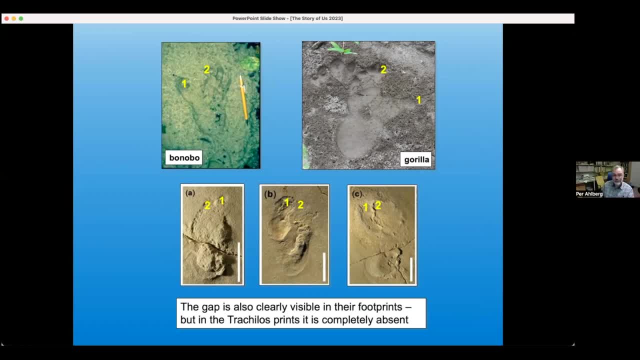 one way or another. What is clear, however, is that you know, while there have been apes in what is now sub-Saharan Africa all along- and that was always a nice, friendly environment for apes- the ape-friendly part of this region of the world used to be much. 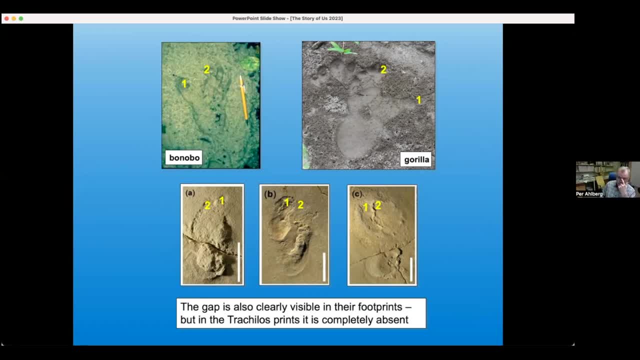 bigger and extending much further north, Right, Right. Well, that makes sense. You know the world is a drastically changing place that we're seeing right now during this sixth great extinction. so, Yep, Yes, indeed, We've made it a priority for now to just somehow 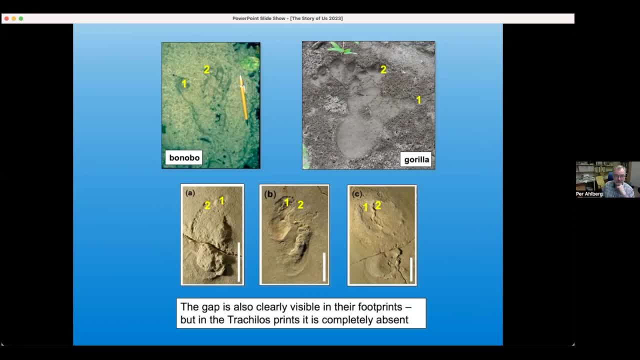 somehow keep the apes that we still have. I mean, you know, there's all sorts of things that we don't want to go extinct, but I think the extinction of any of the great apes would be about as great a tragedy as we could have really both. 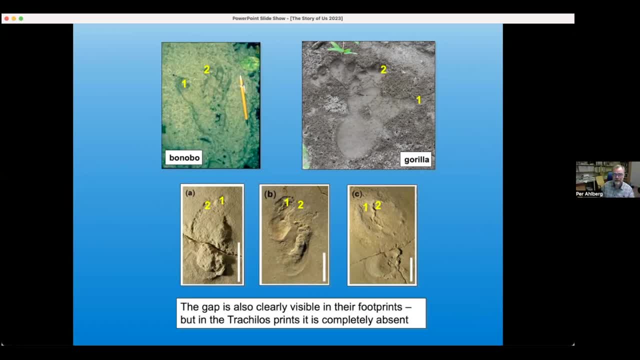 for their own sake and in terms of us understanding where we belong among the animals. I fully believe that and that is why I am unabashedly going to say I am a charity giver to all four great apes, So I think everyone should spend a little time or volunteering. 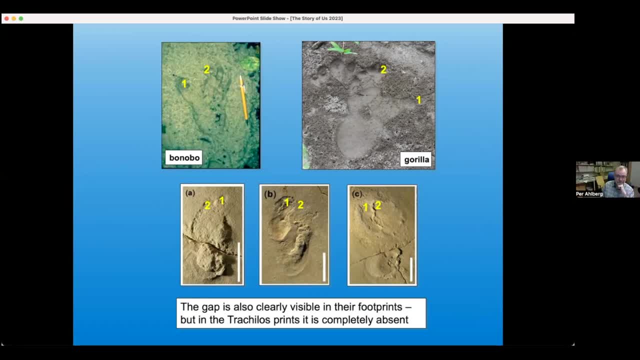 if they can't afford to give to groups working to help these apes survive because the world we've created is not fit for them right now? Totally agree. Well said, And with that I think we will call an end to this interview. 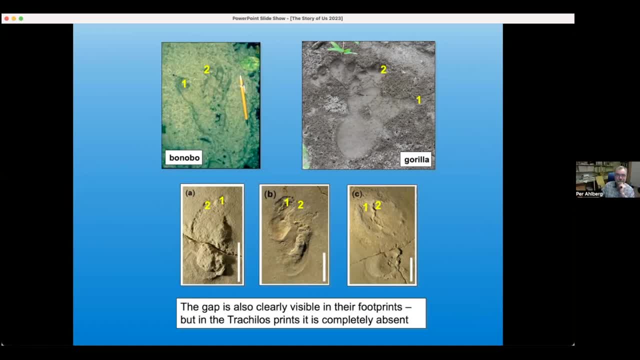 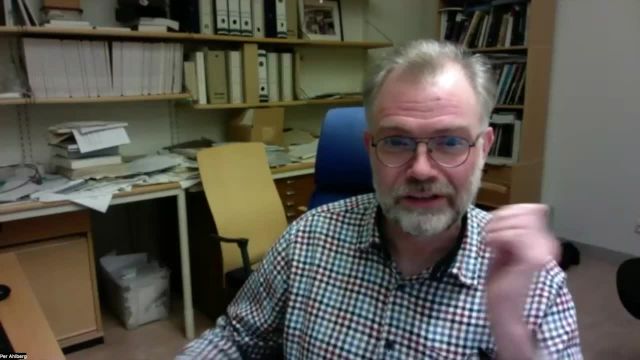 unless there's anything else you wanted to add. No, I don't think so. Well, thank you very much for having me on. It's been a pleasure and really very enjoyable and very interesting. It was wonderful, and I want to thank you so much. 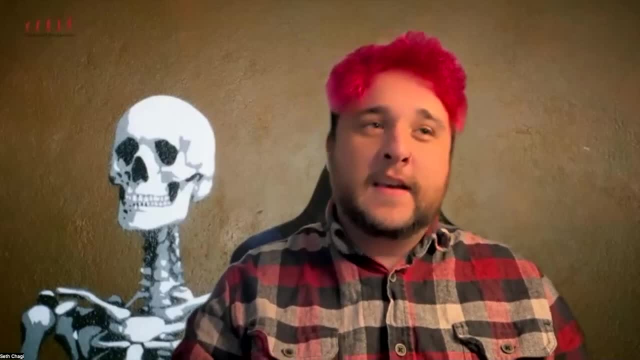 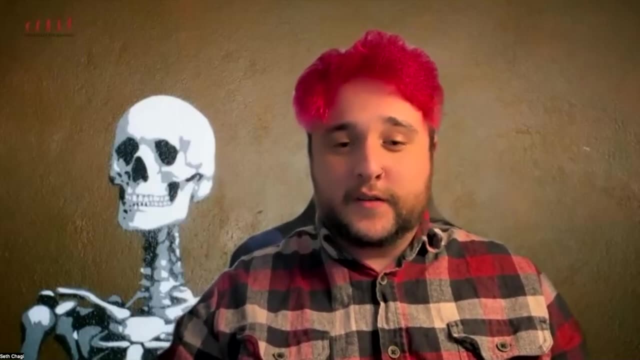 for coming on and taking my invitation, And I just want to remind everyone that I will put contact details at the bottom of the description so you can get those files and see the pictures in high detail and do pretty much what you need with the 3D files.